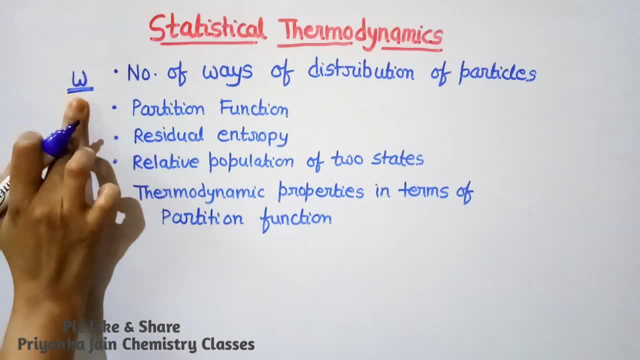 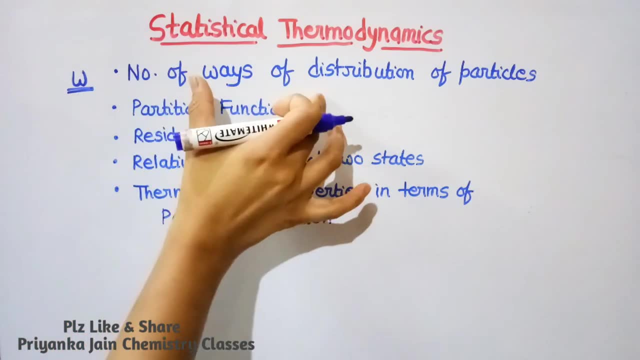 about this w? okay, So you have to find out this one, okay? or it is also called the weight of the configuration. okay, All things are same. we have to find out the number of ways in the case of three different statistics. okay, So, firstly, we will understand this one and we will solve different. 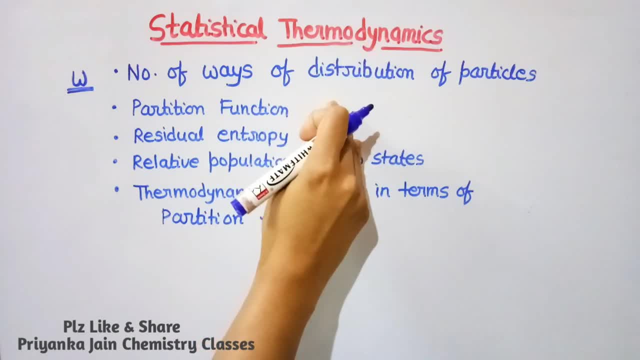 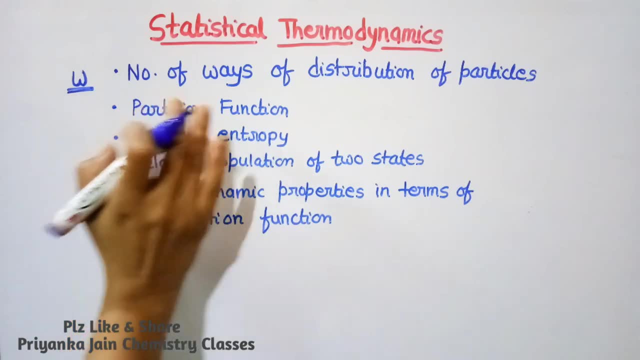 types of questions, What are the different cases, What are the possibilities? Okay, we have to see all the things about this, because this is very, very important. Another thing is the partition function: Three different type of partition functions, and I have already made a particular. 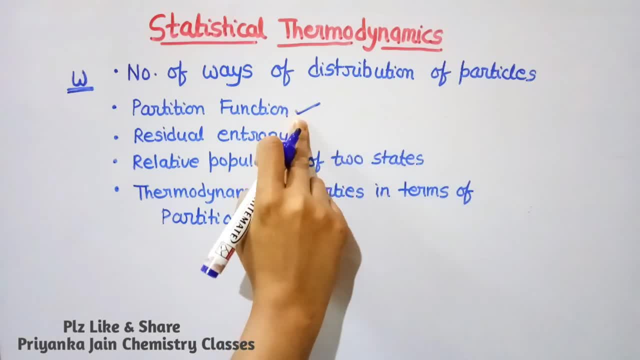 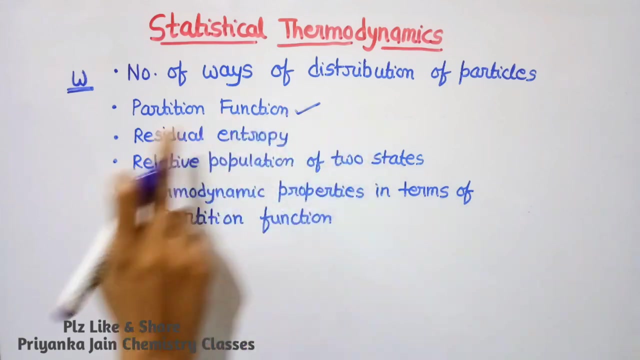 video on this thing. okay, So you can see the link of this video in the description box. Okay, and I have already made a video also on the problems based on the particle partition function. okay, And if some problems are remaining, then I will solve them in the later videos, okay, Next. 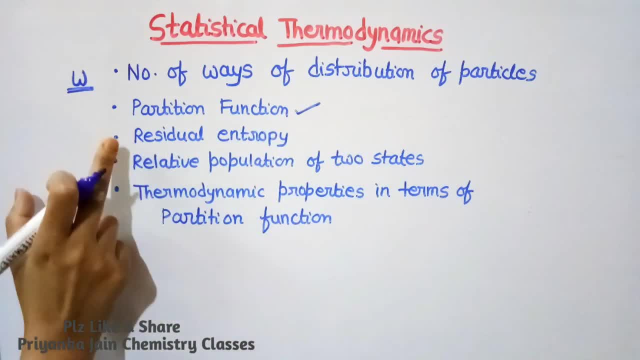 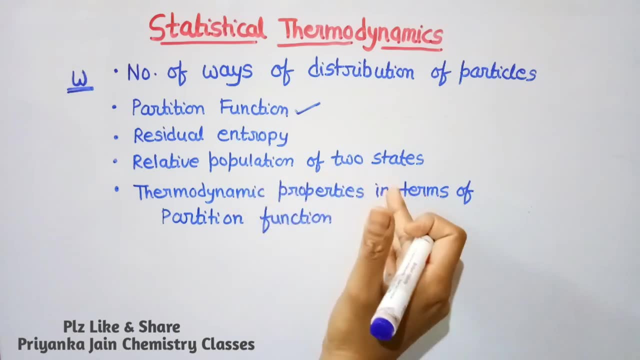 thing is the residual entropy, and it is also very small thing, okay, So we will understand it also. Then there is the relative population of the two states. It means if we have to find out the relative population of excited state and the ground state, then we have to find out the relative. 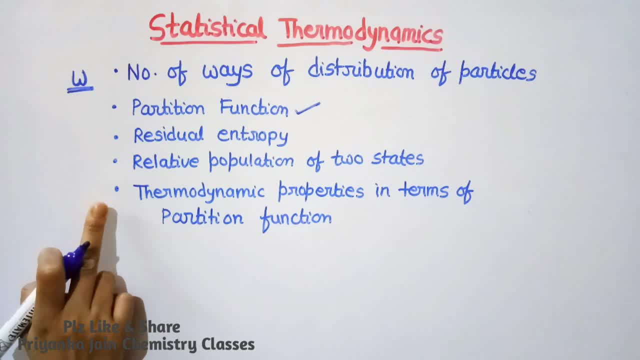 population of the two states. okay, So we will see it. and the next thing is the thermodynamic properties in the terms of partition function. It means the entropy, internal energy, Gibbs, free energy, etc. in the terms of the partition function. So these are the things that we have to study here. 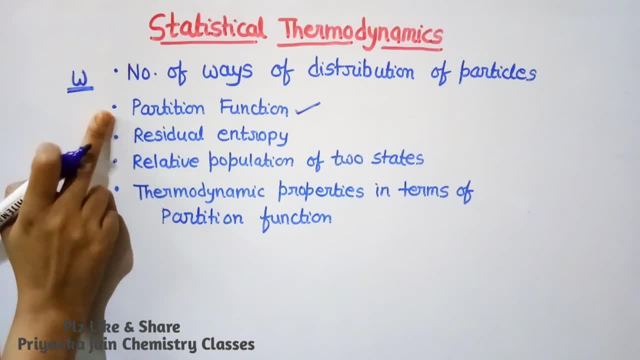 okay, And about the partition function and its problems. I have already uploaded two videos So you can watch that videos okay. So let's start. What is the statistical thermodynamics? Actually, statistical thermodynamics provides a link between the classical thermodynamics and the 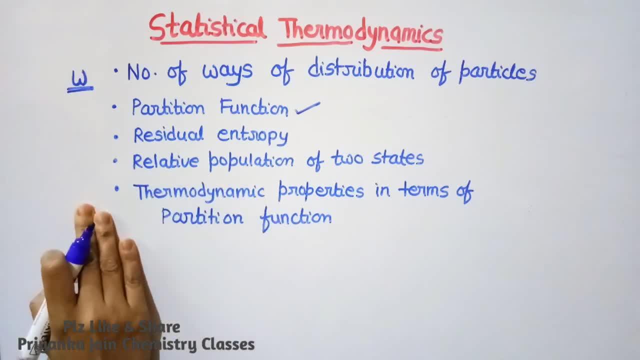 quantum mechanics? okay. In the classical thermodynamics we study about the macroscopic properties. What are the macroscopic properties? Macroscopic properties means temperature, volume, pressure. These all properties of a particular system. We have given a system in this manner. right, This is a system okay. 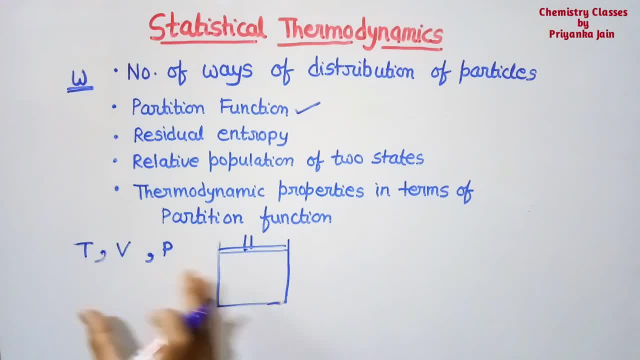 which there is a gas. okay, so we have to see the temperature, volume, pressure, it is of a system as a whole. okay, this is called the macroscopic properties. but what are microscopic properties? we study microscopic properties in the quantum mechanics. microscopic properties means the properties on the particle level, okay. okay, about the microstates. i have already uploaded one video. 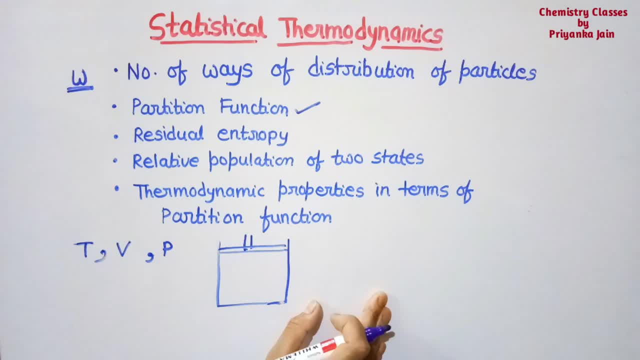 if you want to see the basics of the microscopic properties and the macroscopic properties and what are the microstates, if you want to see the basics, you can go through that video. i have already uploaded a video on the microstates, okay, so you can watch that video. okay, i will give you. 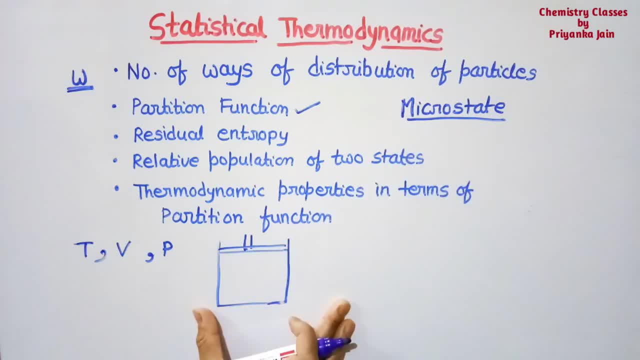 the link. okay, so here we have to see these all things, okay. so one thing was that okay. now come to our first point, that is, number of ways of distribution of particles. this is the thing that we have to find out, and this is also known as the thermodynamic probability, and for finding this one, we should know about the particles. 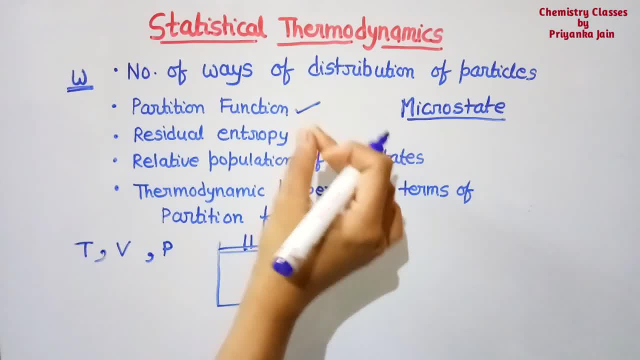 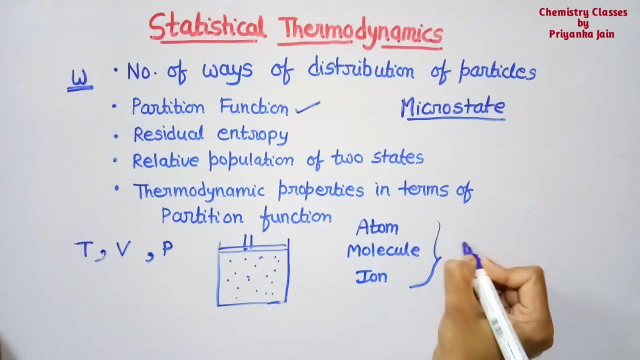 actually in the statistical thermodynamics we consider the particles. particles are what it means: any atom or any molecule or any ion, anything that we have given that is filled inside this piston. okay, inside the system. okay, that is making a unit. this all are called here the particles, okay. 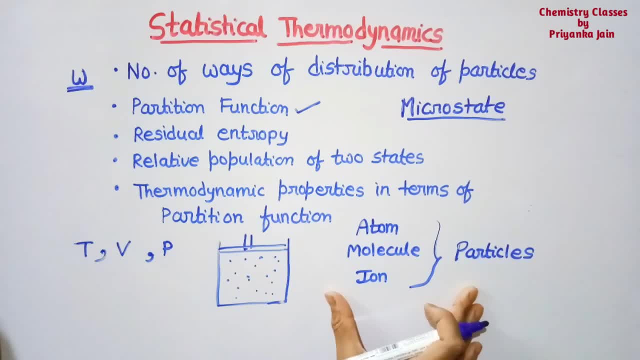 these all are considered as the particles in the statistical thermodynamics, okay, and we have to distinguish between them. they may be distinguishable or non-distinguishable. for this, there are three different statistics and we have to consider them, okay, so, firstly, we will see these three statistics. okay, so there are three different statistics that we need to understand. 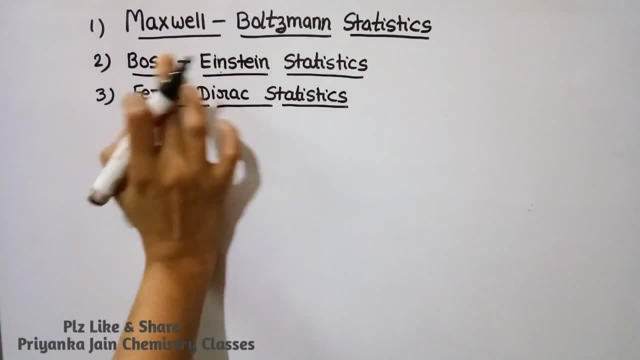 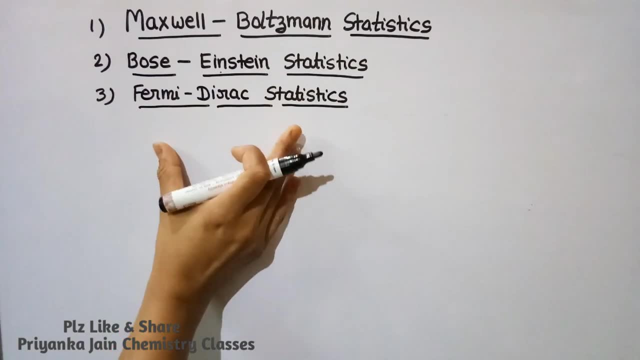 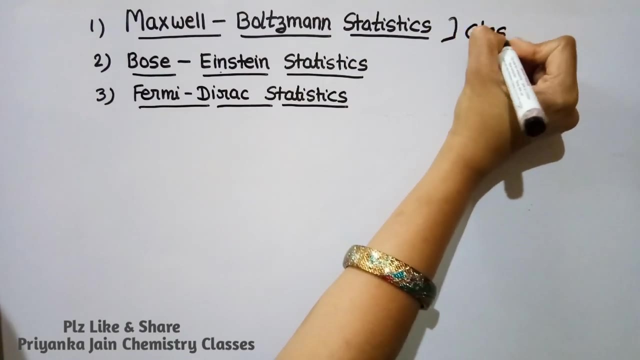 statistics: one is the Maxwell Boltzmann statistics, another is Bose Einstein statistics and third it's the Fermi direct statistics. okay, all of them are very, very important. so this Maxwell Boltzmann statistics is actually known as the classical statistics. okay, and these two are actually based on the 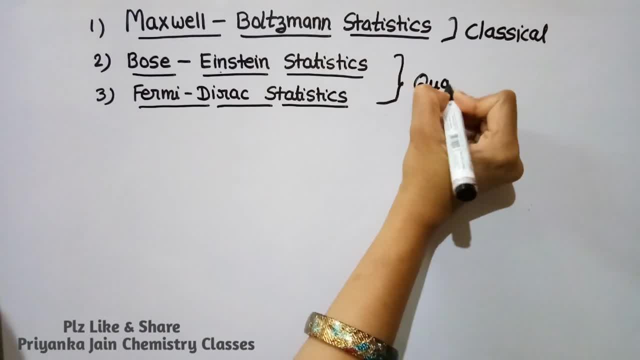 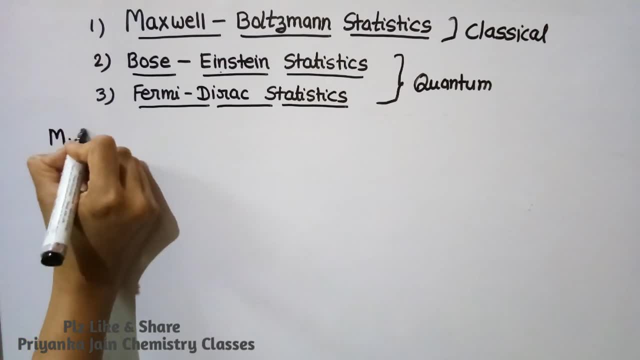 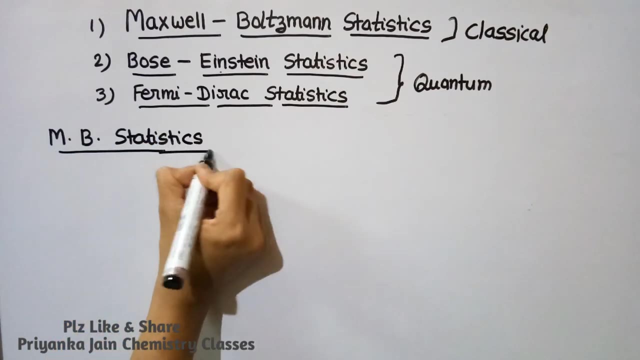 quantum mechanics, so these are known as the quantum statistics. okay, so firstly we have to see the Maxwell Boltzmann statistics and this we can also write as MB statistics, okay, so the basic assumptions about this that we have to study here is what? first thing is that here the particles are assumed to be. 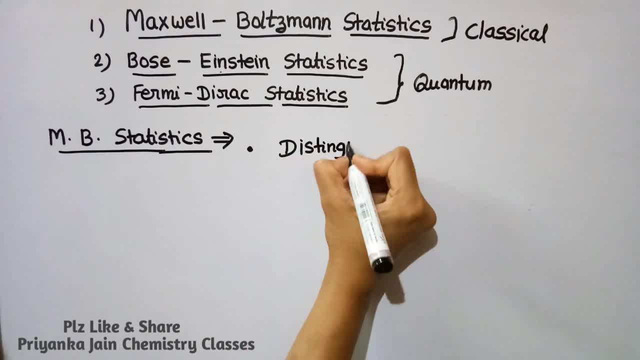 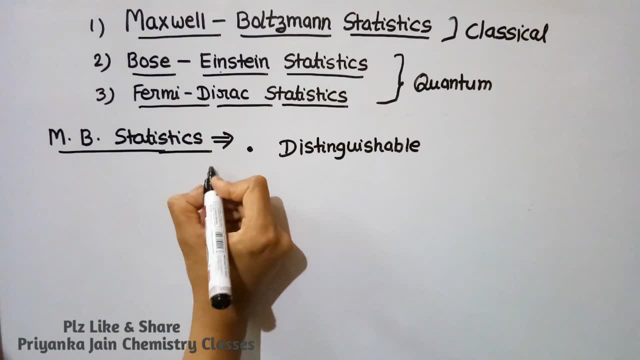 distinguishable. what is meant by distinguishable? it means we can identify them. okay, if we have given three different particles, these are the three different particles, then we can identify them. okay. suppose this one is like this: okay, and another one is in this form: okay, so we can distinguish between them. okay, so these 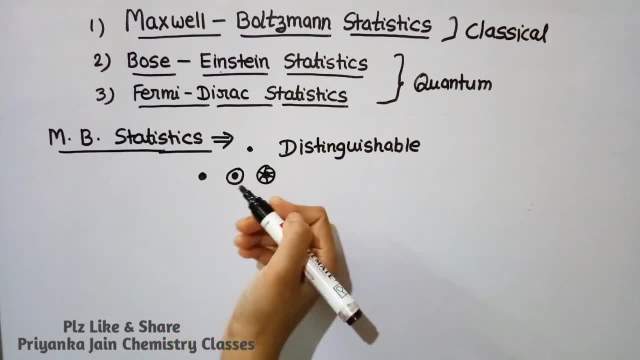 particles are distinguishable particles. okay, so we will name them. this is a, another is b, third one is c. okay, so these are distinguishable particles. another important thing is what? another thing is that there is no restriction on the particles. it means any number of particles can occupy the 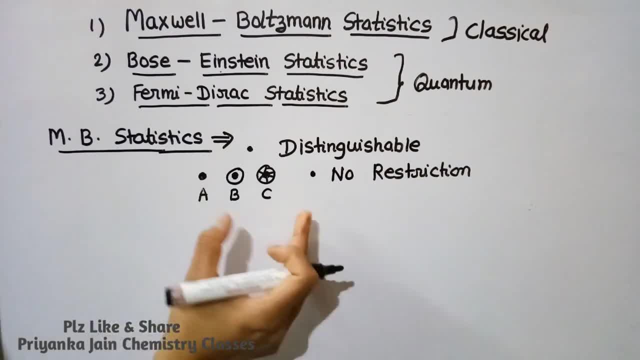 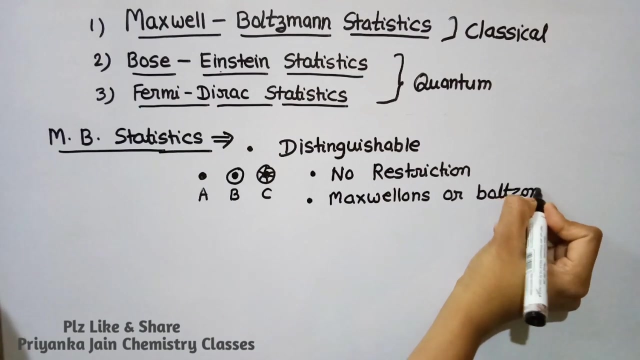 energy levels. okay, either one can occupy, or two can occupy, or all the three can occupy the one energy level. so there is no restriction on these particles, okay, another important thing is that these particles are known as the Maxwellians, or voltoids, volts on. okay. okay, these particles are named as max balance or pole Jones. okay, so see here, suppose. 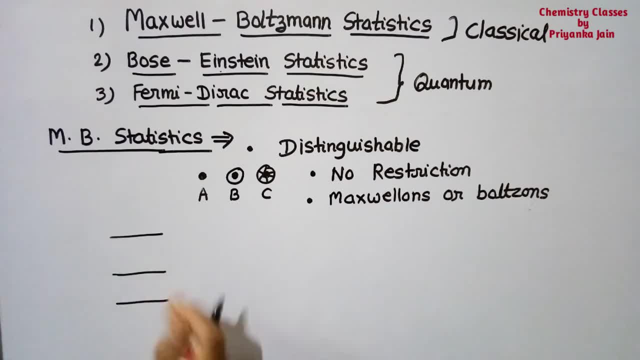 we have three energy levels in this way, okay, and we have given these three particles. now, these three particles, how we can fill them? suppose there may be two particles in this level, or one can be. this way, for example, we can fill them with. sometimes we can fill it with more particles, but we don't. 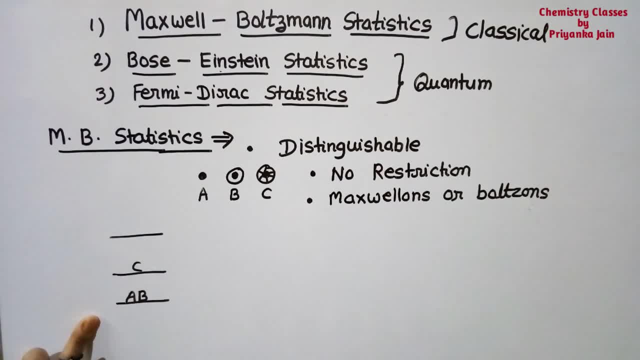 in this level. okay, now these particles are distinguishable. okay, we can distinguish between them. so there may be another condition that this A is in this level and these BC are in this level. right, there may be another condition: this B is in this level and remaining one is A and C that are in this level, or? 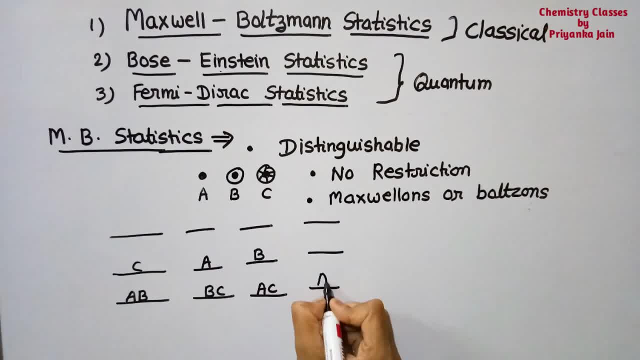 there may be another. conditions, all are in different levels. ABC in this way, okay. or these may be in the different woods, okay, here may be. here may be B, here may be C. so there may be a number of ways. because these particles are distinguishable, okay. so there may be a number of ways for filling them. so we 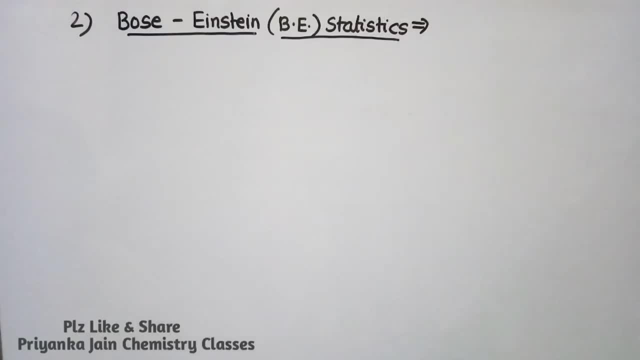 have to consider them also, okay. okay, now see the another statistics, that is, Bose-Einstein or BE statistics. what are the key points of it? okay, so see here. the first is point is that the particles are here indistinguishable. okay, the particles are indistinguishable means we. 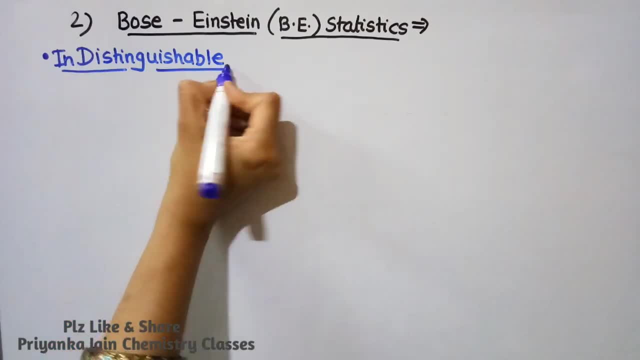 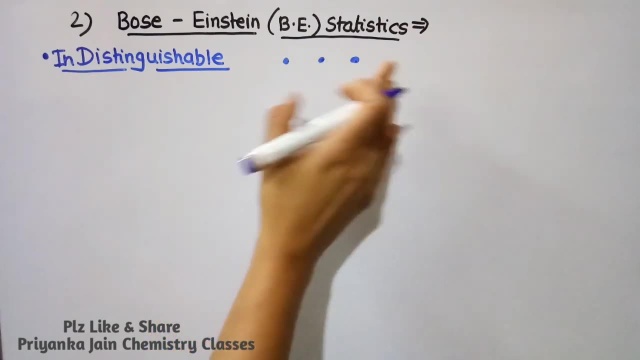 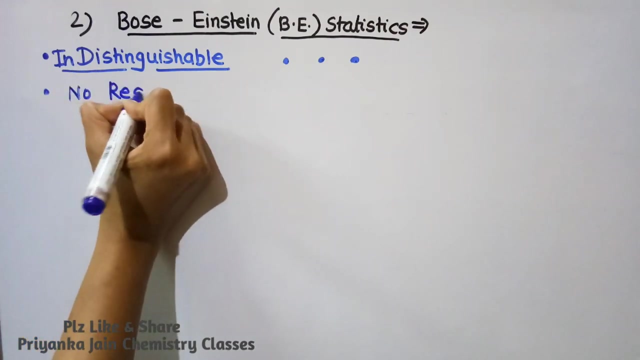 cannot identify between the particles. okay, it means in this way, these are the particles, we cannot identify them. what are? which is a, which is B? okay, all are same type, right. and another thing is that there is no restriction on the particles. it means any number of particles can occupy any energy level. 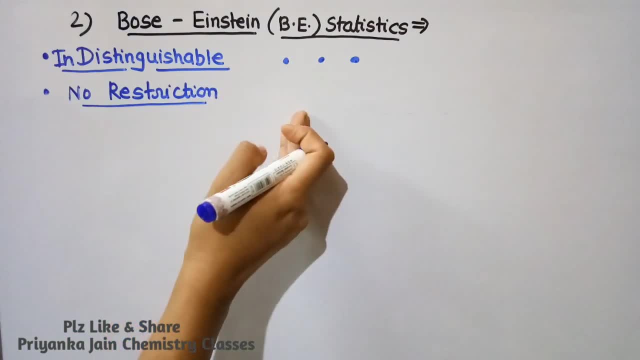 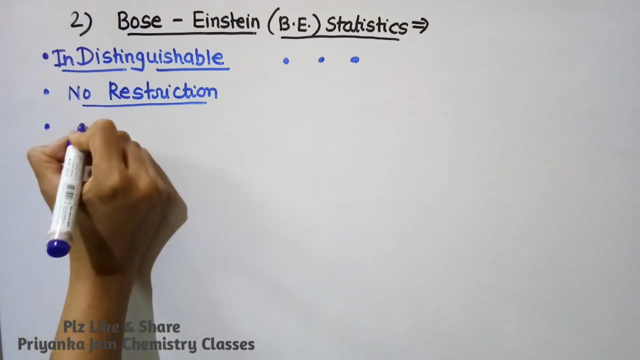 okay, this thing is same as that in the case of the Maxwell Boltzmann statistics. here, the difference is what these particles are indistinguishable, while there was a particles distinguishable, right. okay, now see. the third thing about this statistics is that the particles here are having the 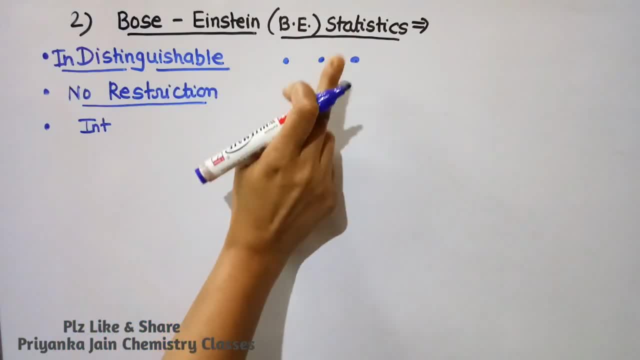 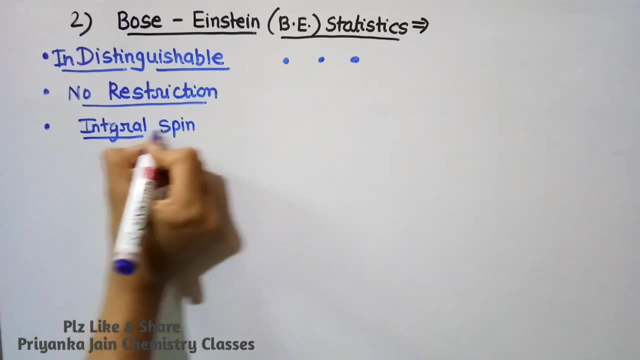 integral spins. this statistics is obeyed by the particles that will have the any number of the spin spin values we have studied in the NMR spectroscopy's we do. it means integral spin, means the spin value may be 1 or it may be 2 in this 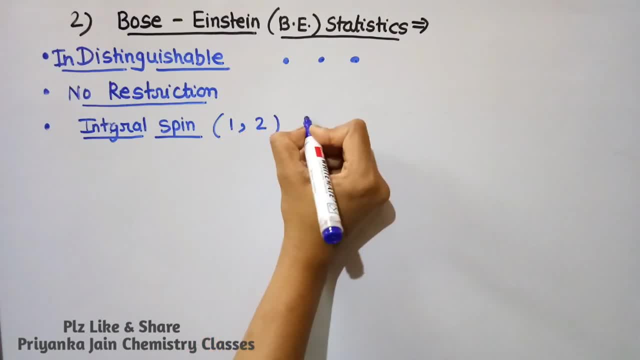 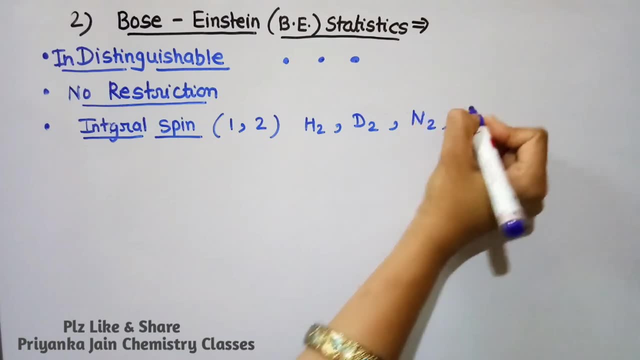 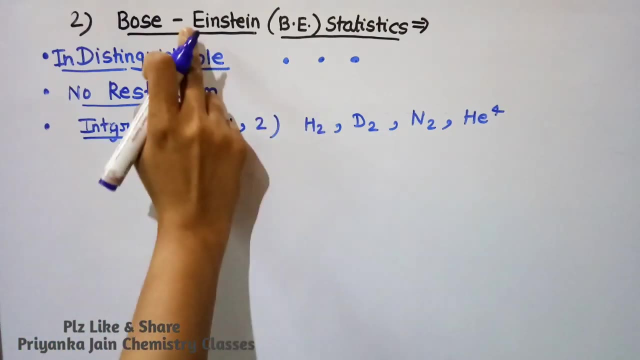 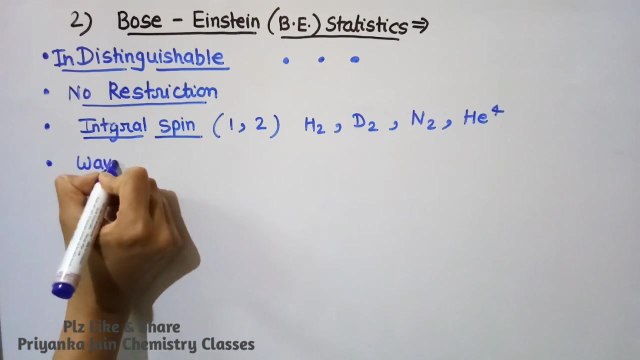 way right. such type of values, for example, in the case of h2, like d2 in the case of n2, okay. or helium-4. these all are the examples of the integral spins, right? so this all will follow the Bose-Einstein statistics, right? fourth point is that here, in this case, the wave function will always be integral spin. 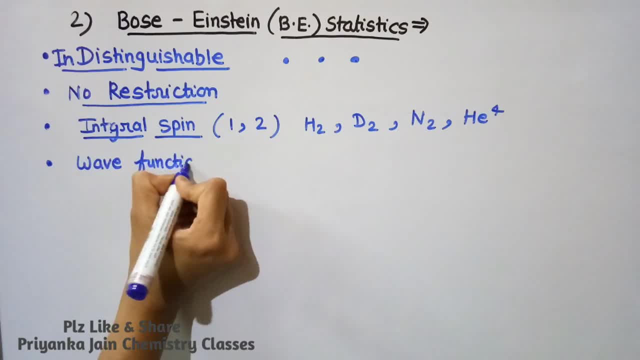 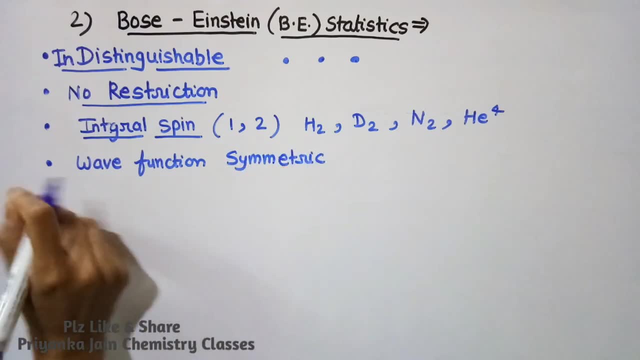 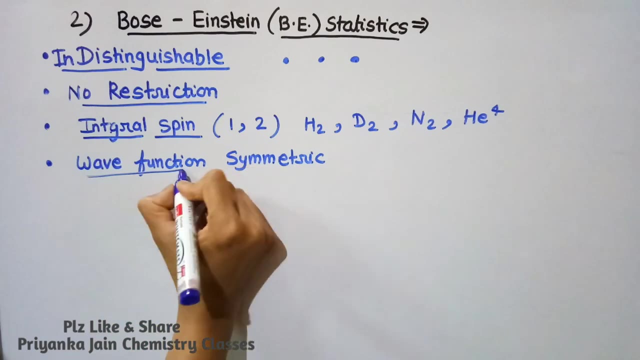 symmetric. we have studied this term in our video of the quantum mechanics. I made one video on the Slater determinant. if you have seen that video, I have already told you what is the anti symmetric and symmetric wave function. okay, so see, a symmetric wave function means if we are interchanging the 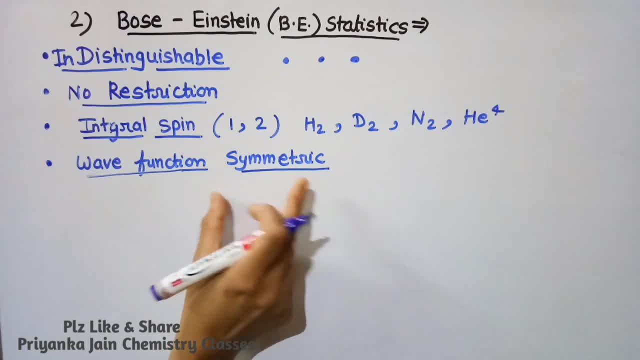 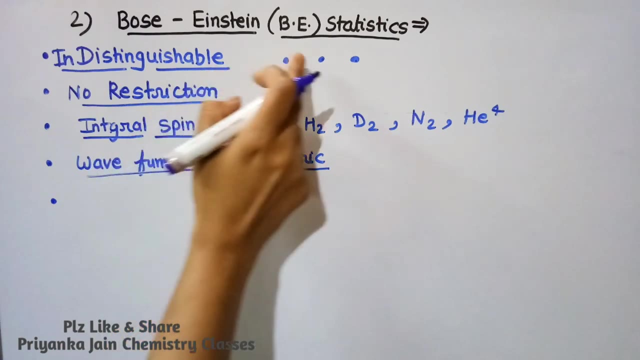 particles. okay, if we are interchanging the particles, then the wave function. if it is not changing the sign, if the wave function does not changes the sign, then it will be symmetric wave function and in this case the wave function is always symmetric. right, okay, now see the last thing. such type of particles are known as the bosons. okay, so in 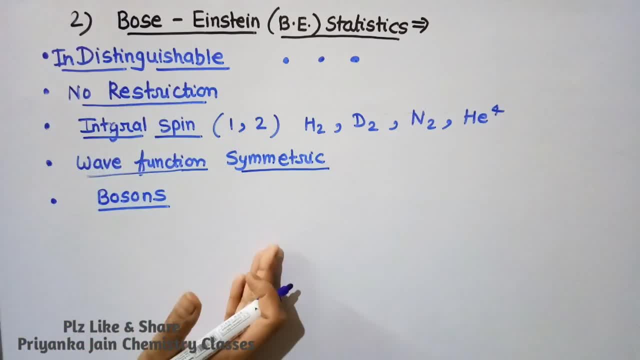 question papers. you may have given that the particles are indistinguishable, or you have given that they are following the boson Einstein's statistics, or they may give that the particles are bosons, or they may give that the wave function is symmetric in any other type they can give you. 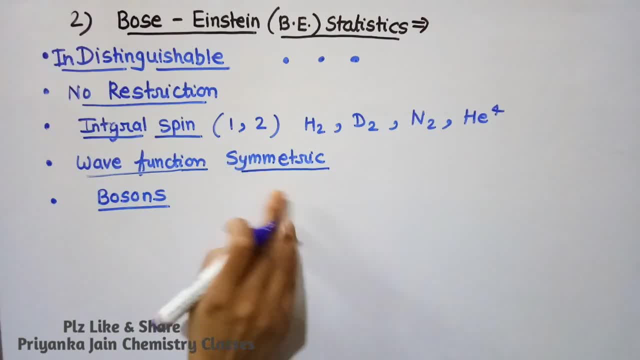 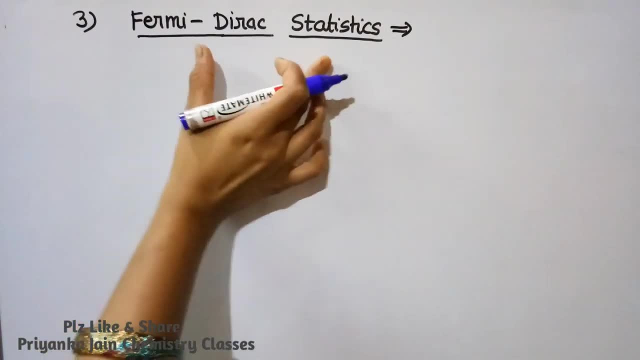 in the question paper, right? so you have to find out the number of ways, and that we will see somewhat later. firstly, see this thing. okay, now see the third type of the statistics is the Fermi direct statistics. and what are the key points here? first key point is that the particles. 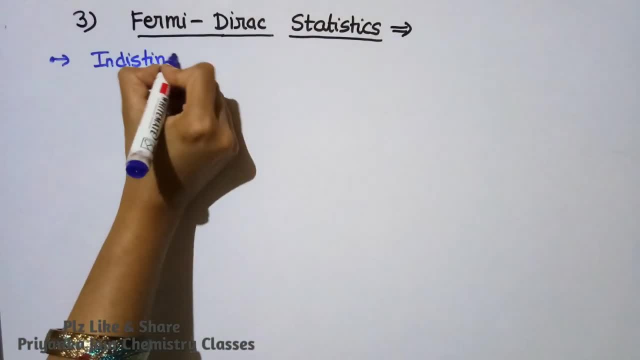 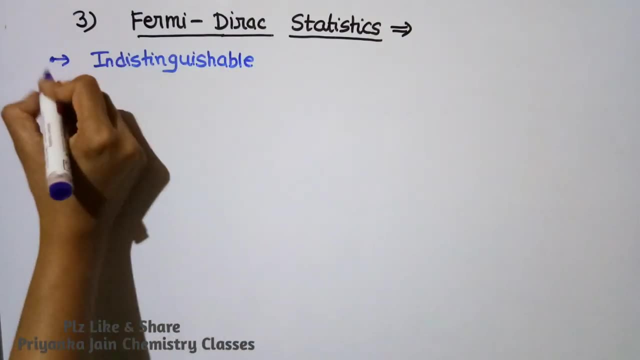 are here indistinguishable. okay, same as we have seen in the case of boson, Einstein's statistics. it means we cannot identify between the particles right. another thing is that here is a restriction on the particles. it means you have to find out the number of waves, and that we will see somewhat later. firstly, see this thing. 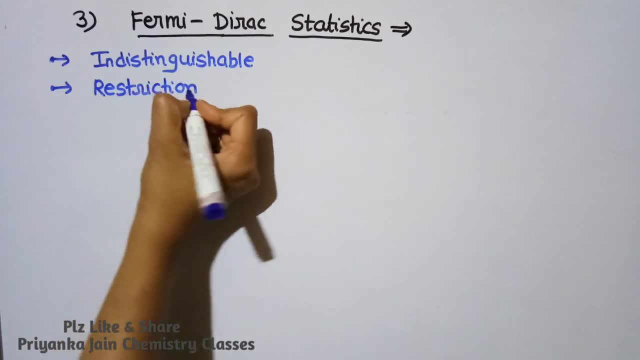 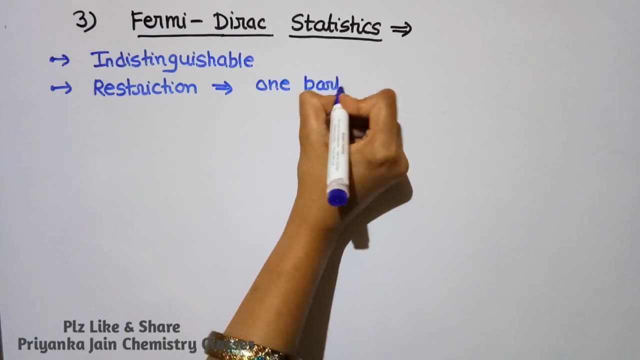 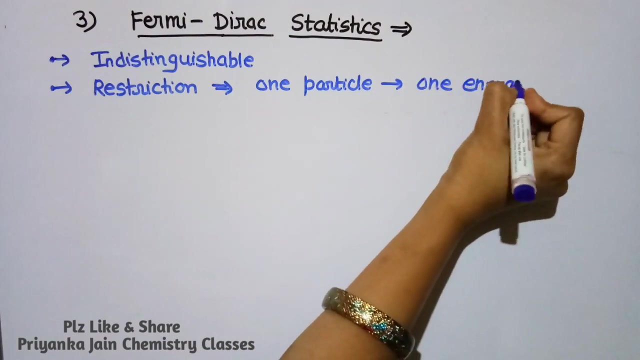 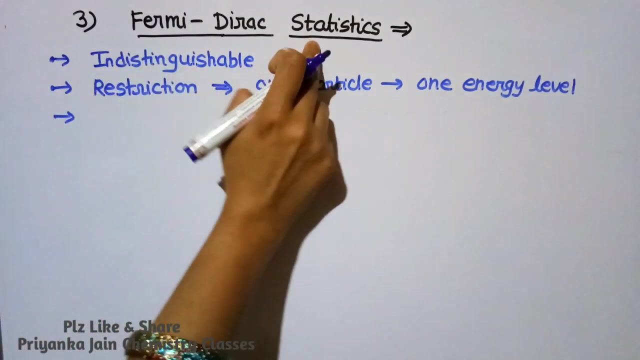 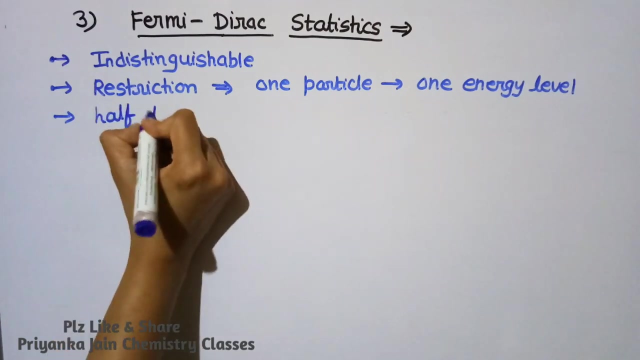 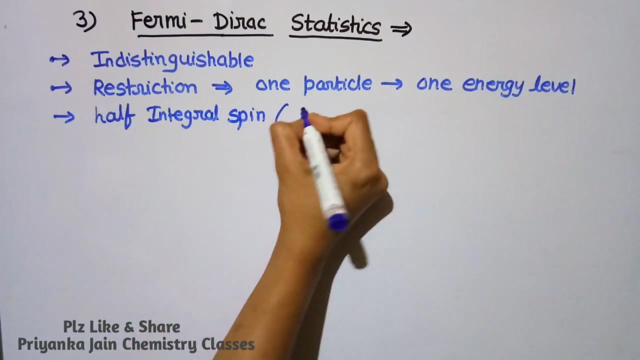 only one particle can occupy one energy level. right, that is a restriction here. one particle will occupy one energy level, right, okay, now see the third thing here. this statistics is obeyed only by the particles that will have the half integral spin. what is meant by half integral spin? it means the spin may be either half or it may be three by two. 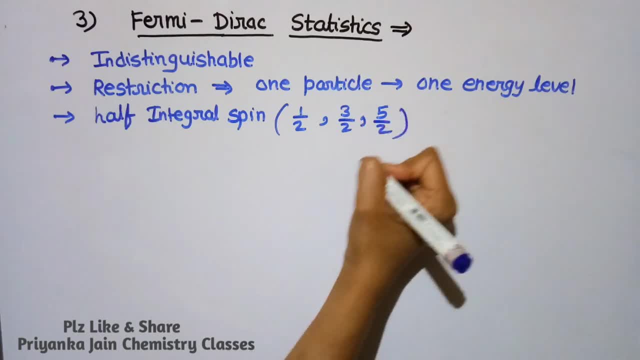 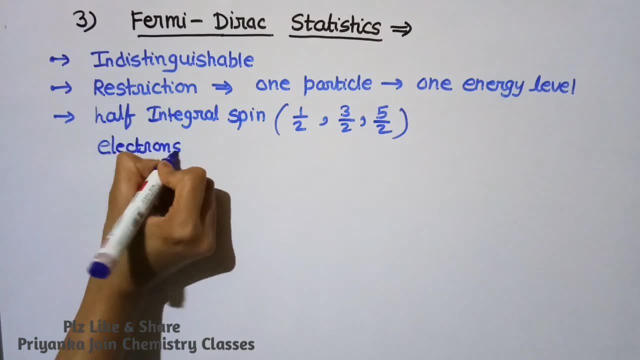 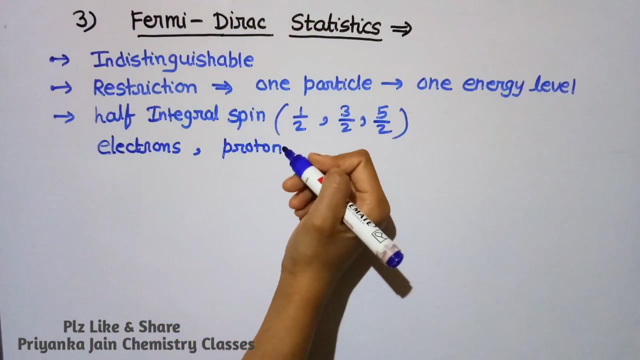 or five by two. it means in this way: right. so this is obeyed by the particles, like we have given electrons, okay, or we have given the protons. in all such cases, they will obey the Fermi direct statistics. okay. so this is obeyed by the particles, like we have given electrons, okay, or we have given 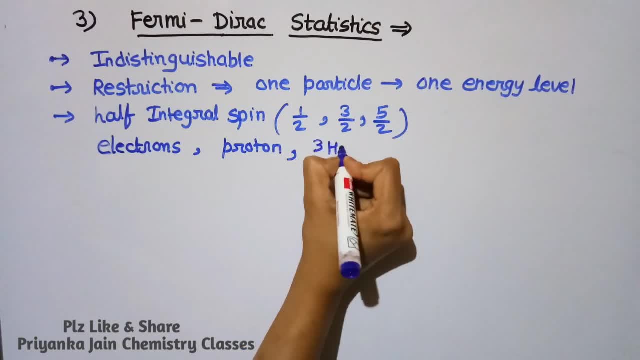 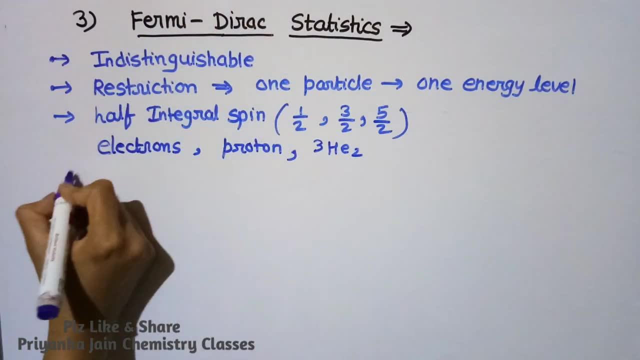 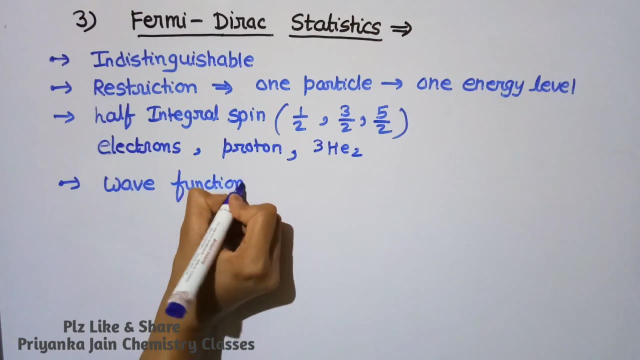 electrons over to rank, or they have given of us three and G two in this way. okay, right, so all in these cases we will see the Fermi Direct statistics. and all the thing here is the action is always anti symmetric. and what is meant by the anti symmetric wave function? it means, if we 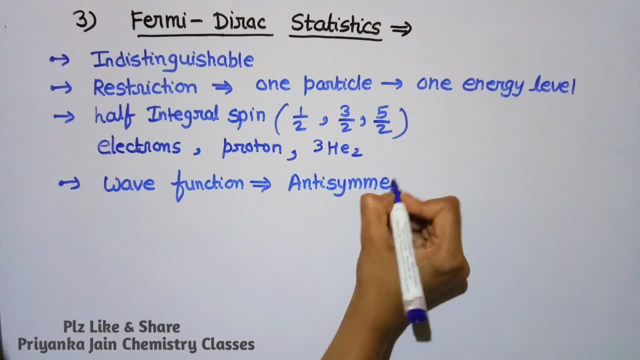 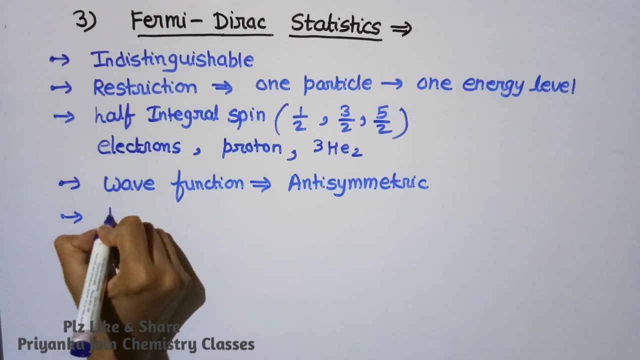 are interchanging the particles nanned up. a function will change its sign. okay, and last thing is that such types of wave functions will always iht to the fact that if the wave tenemos type of particles are known as fermions, okay, so if you have given the fermions, it means the 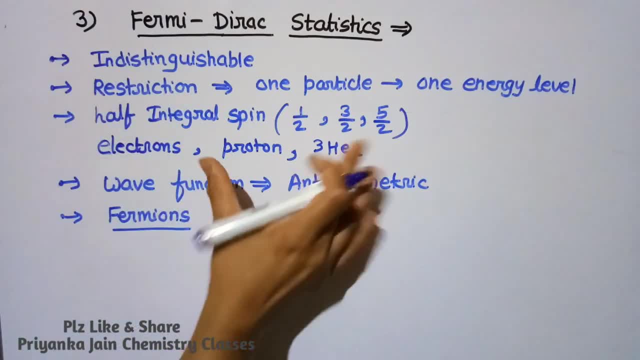 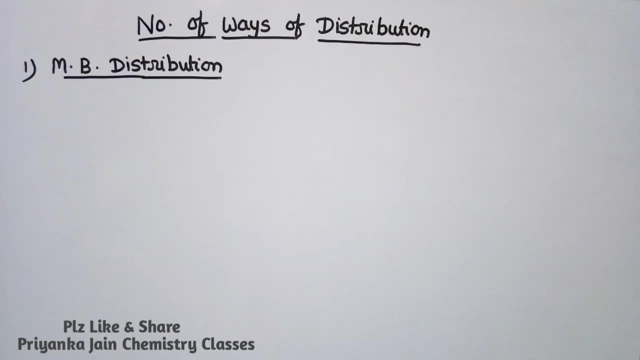 particles are indistinguishable. there is a restriction that only one particle can occupy one energy level. okay, okay, now we have to see the number of ways of the distinguishable of particles. it means we have to see the thermodynamic probability or we have to find out here the w. 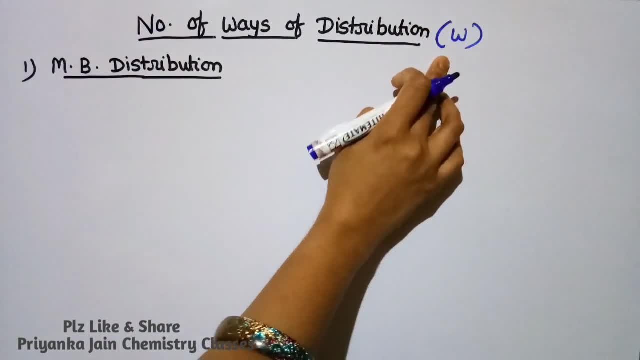 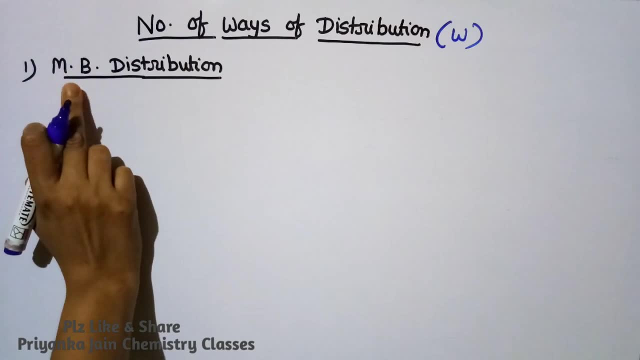 that is the most important thing that is asked in the question papers. okay, so there are a number of cases and we have to see all of them one by one. first thing is we have to see the for the mb distribution. it means maxwell boltzmann distribution when the particles are given to us. 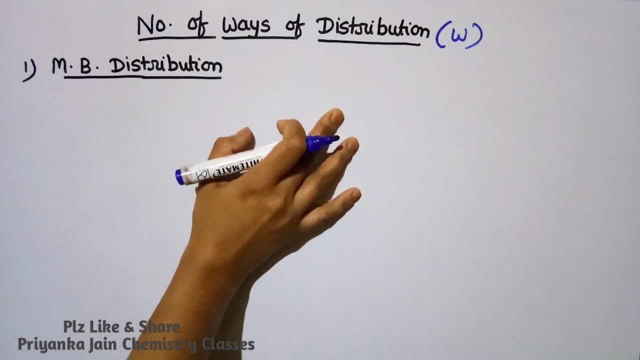 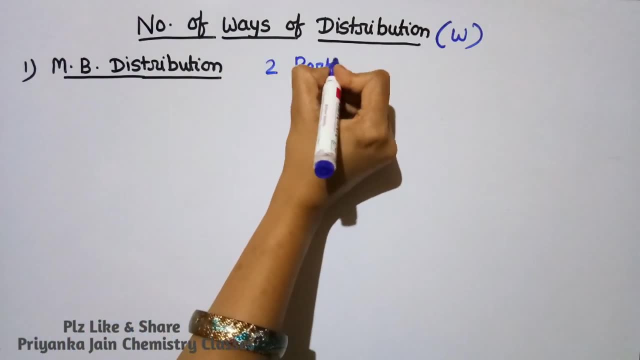 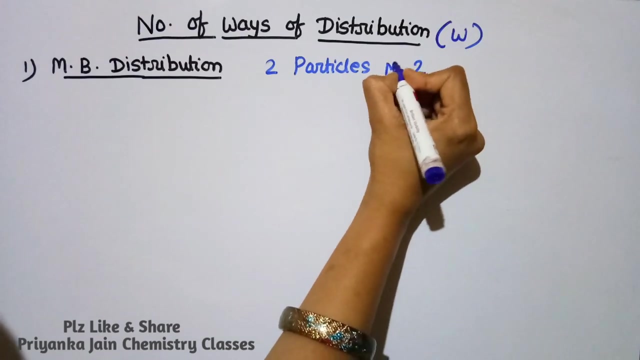 are distinguishable and there is no restriction on the particles. okay, so the first case is the simplest one. suppose we have given two particles. okay, we have given two particles and the energy levels are also two. it means the value of m is equal to two and number of particles? it means 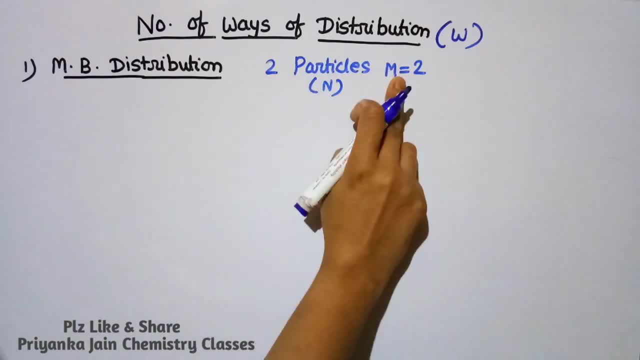 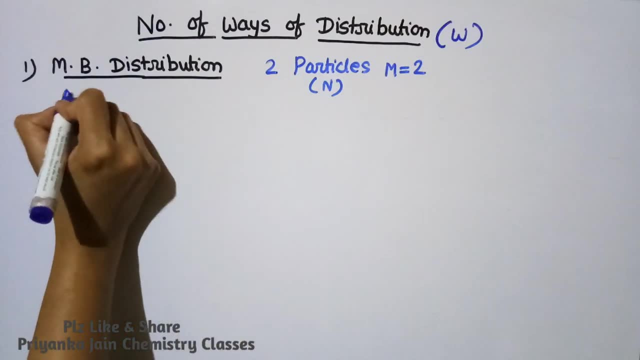 n is also equal to two. n is the number of particles and m is the number of states. okay, so see here, if we have given two particles, it means we can name them because they are distinguishable. suppose one is a, another is b. okay, now see here, there are two energy levels. 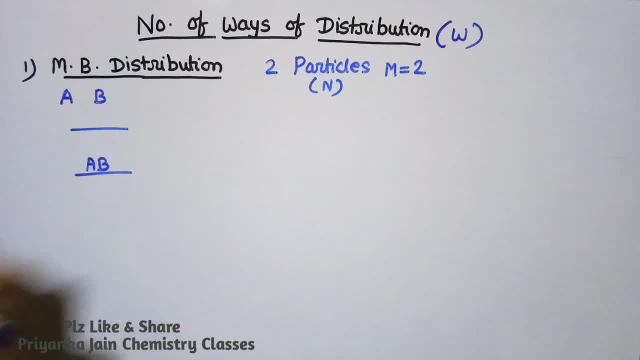 now, what is the condition? one may be that both are in present in this level. okay. another condition may be: both are present in this level right now. another condition may be: one is present here, but the particles are distinguishable, we can distinguish them right. so there may be another. 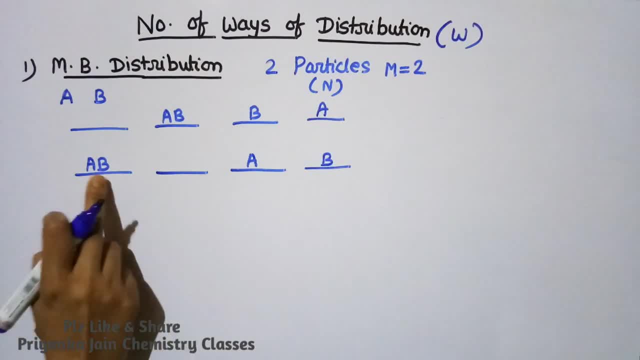 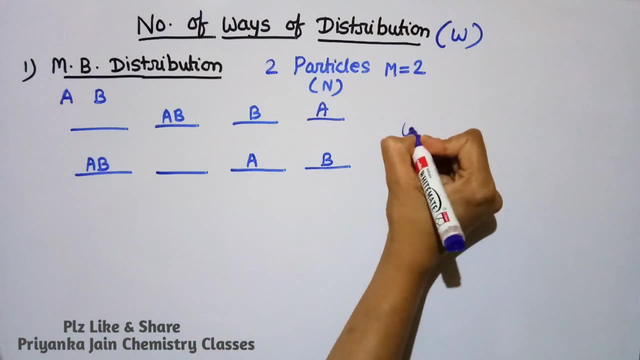 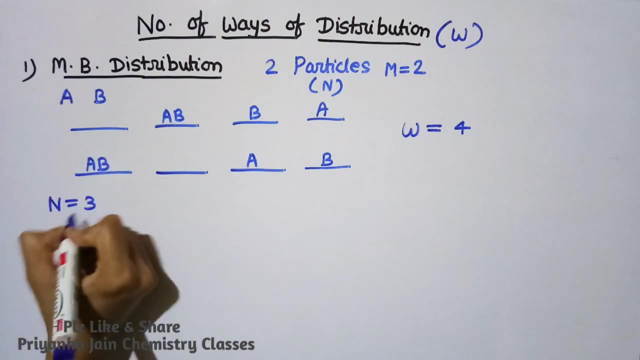 condition that a is present here, b is present here, right? it means there are four different ways by which we can distribute these two particles in two energy levels. so number of ways is equal to four in this case. right now, suppose we have given three particles, okay, and the number of states is: 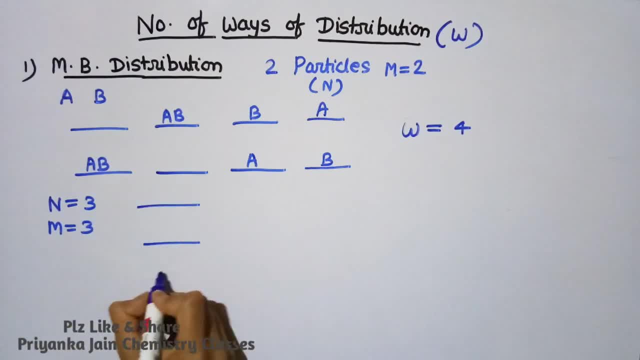 also equal to three. okay, now there are three different states and three different particles: a, b and c. there may be a number of ways here. okay, suppose one is here. a is here, b is here, c is here. okay, another condition may be: c is here, b is here, a is here. 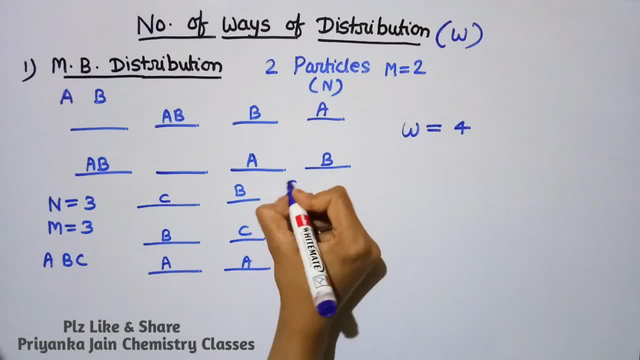 okay, there may be a lot of conditions here. suppose c is present here and a is present here, b is present here, or there may be a condition that a, b is present in this and c is present here. so there may be a number of ways and we cannot find them. 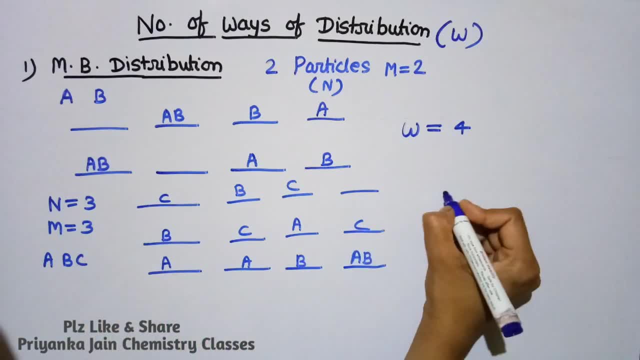 counting them. okay, so here is a formula for this. what is the formula? if we have given such type of simple case, then we have to use this formula. it means w is equal to m to power, n. okay, so in this case, value of m is 3, okay, number of particles is 3, right, so what will be condition here? 3 to power. 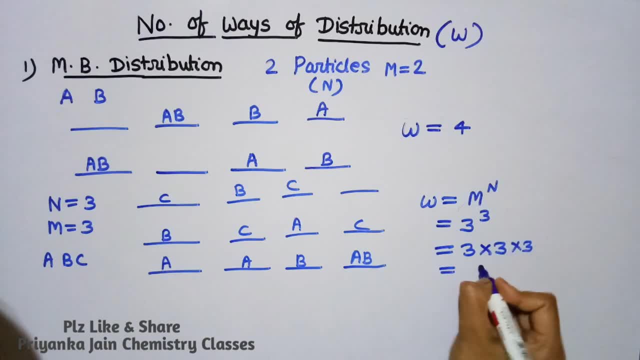 3. it means 3 into 3 into 3. so there are 27 ways to distinguish, distribute these particles between these three energy levels. okay, so we have to apply this formula, okay, in these type of simple cases. so this is number one formula, right? okay, now see the condition number two. if we have a restriction here, 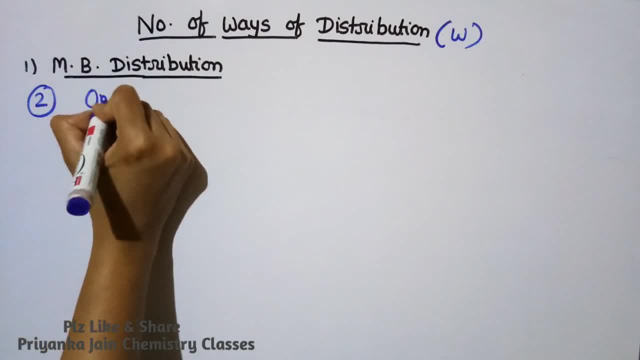 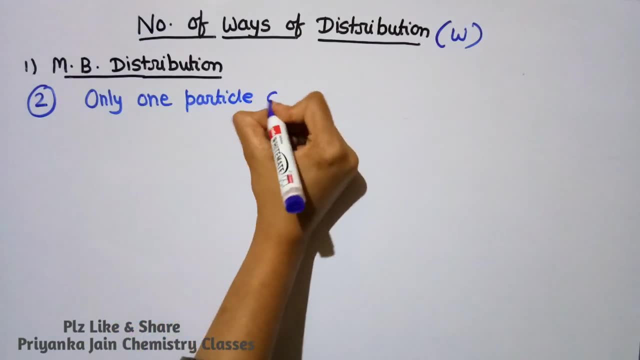 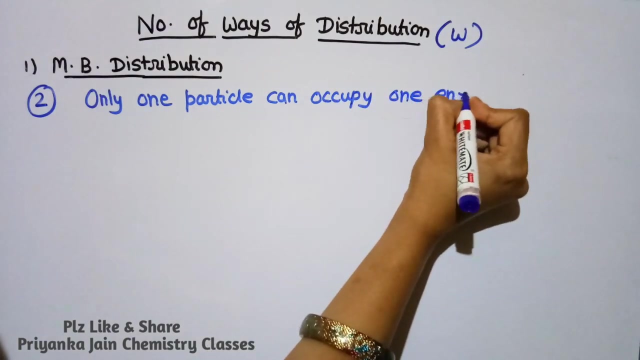 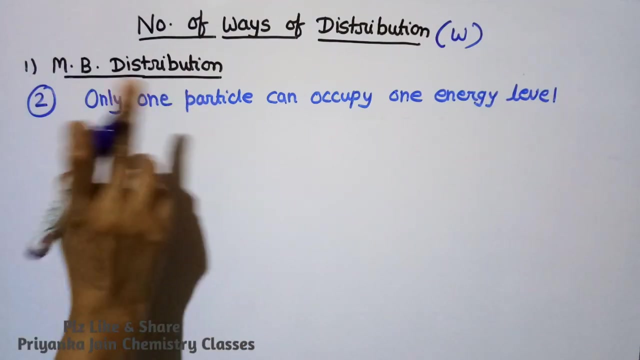 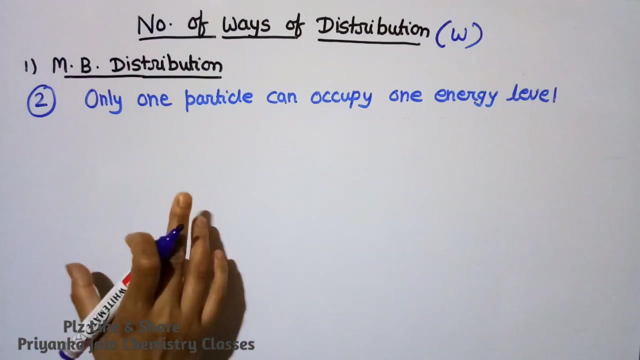 suppose we have given a restriction that only one particle can occupy one energy level. we know that in the Maxwell Boltzmann distribution the particles are distinguished well and there is no restriction on them. but in question papers may give us the restriction they may give that the one particle can occupy only one energy level. then in such cases 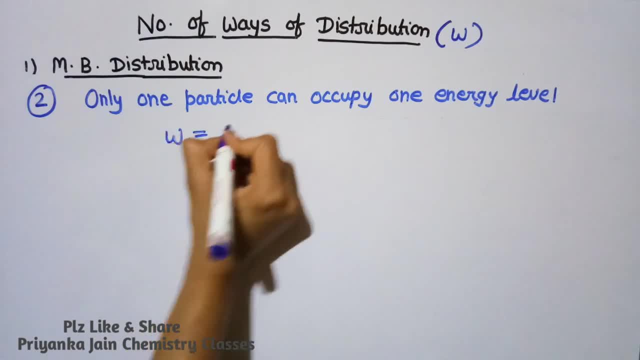 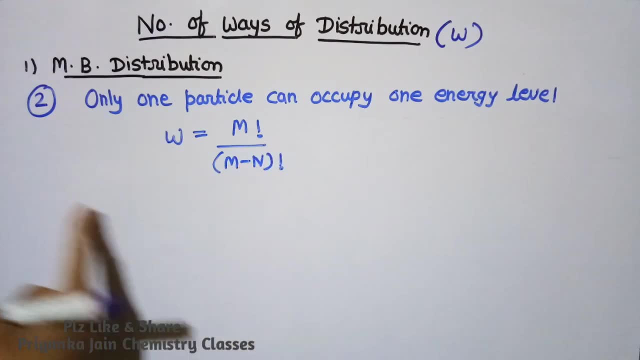 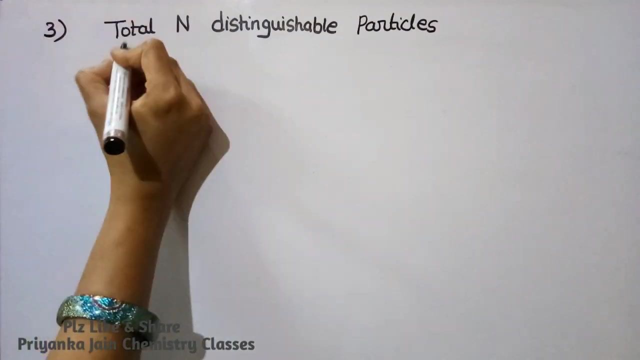 we have to use this formula, that w will be equal to m factorial divided by m minus n factorial. Okay, now see the third condition, when the total number of distinguishable particles is n and there is a condition that n naught particles are occupying the energy level. 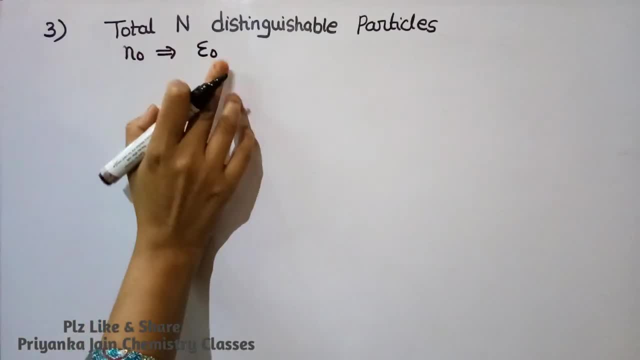 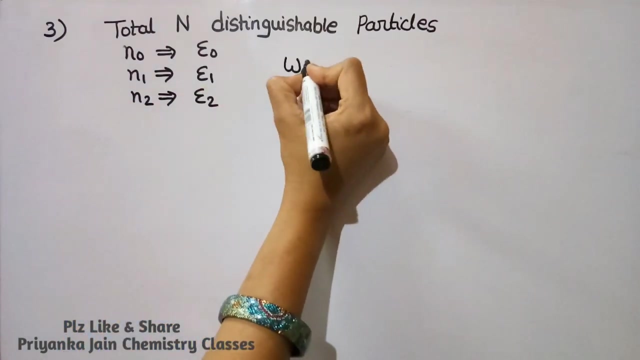 E1, n? naught particles are occupying the energy level E? naught and n1 particles are occupying the energy level E1. Okay. similarly, n2 particles are occupying the energy level E2 in this way: Okay, so in this case the number of ways is given by n factorial divided by n1 factorial. 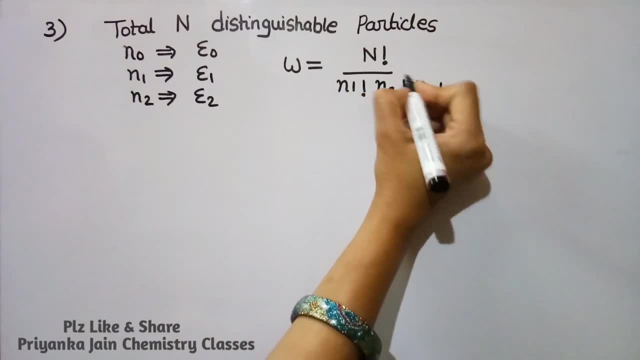 n2 factorial, n3 factorial. in this way, Okay, or we can say this: if we are writing it mathematically, then we can write in this way: w will be equal to n factorial, pi, i, n i factorial. It means this: pi. 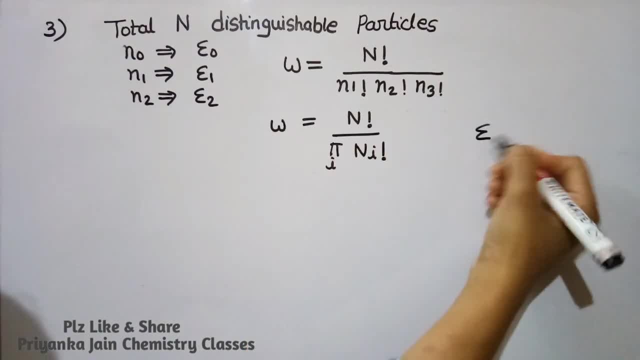 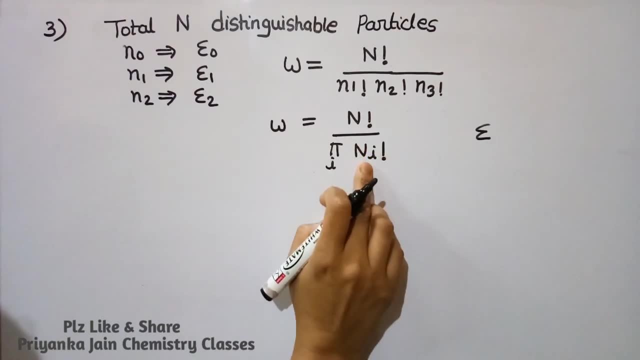 this pi means multiplication. As we know, this summation means the sum of all the terms. Similarly, this pi means multiplication of all the terms Here. n i is what? n? i is the number of particles in any individual energy level. Okay, so we have to do in this. 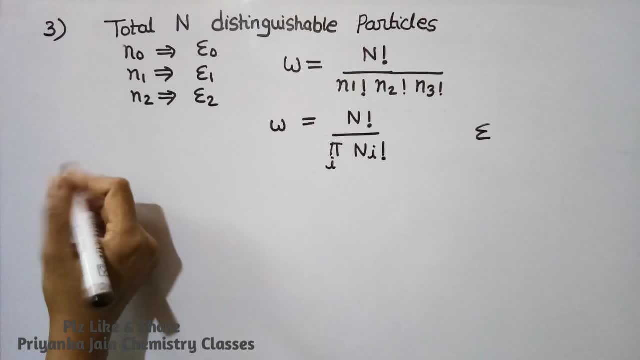 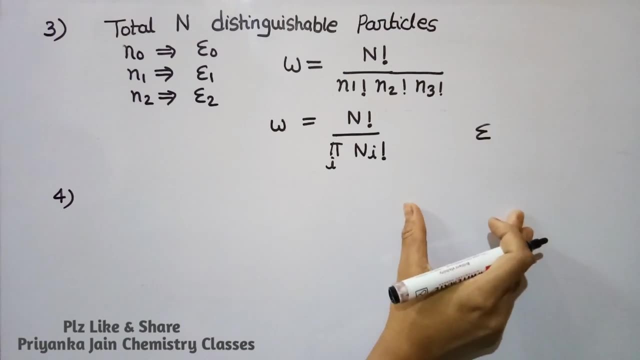 manner. Okay, now see the fourth condition. Fourth condition is when the energy levels are degenerate. What is meant by degenerate energy levels? It means more than one energy levels will have the same energies. Okay, suppose we have one energy level, E1.. 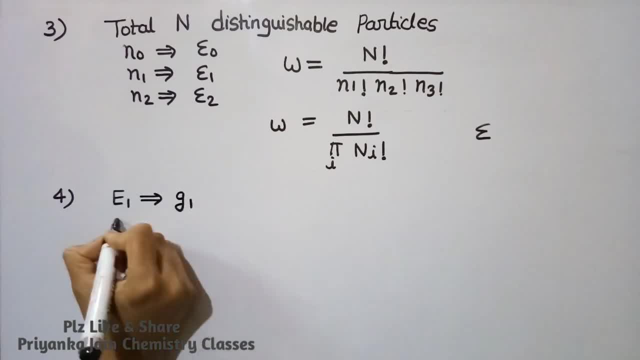 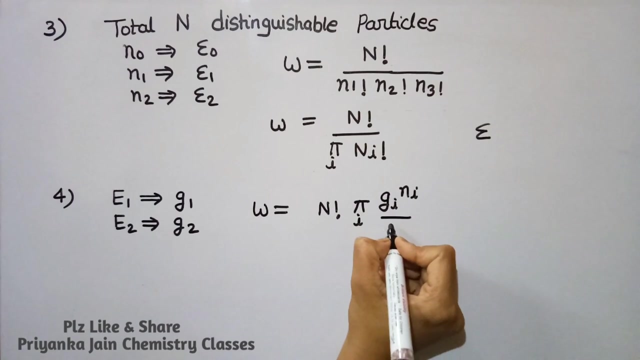 And its degeneracy is g1.. Similarly, another level is E2 and its degeneracy is g2. in this manner, Okay, so what we have to do here, The number of ways is then given by n? factorial and then pi i. It means multiplication of g? i to the power n? i divided by n? i factorial. Okay, this is n? i. 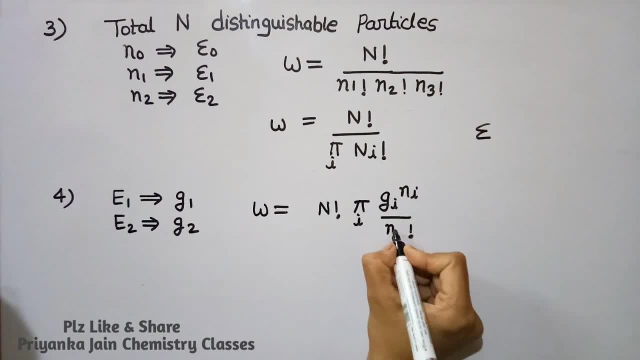 Okay, so suppose we are taking this one case, when E1 levels have the degeneracy g1, E2 levels have the degeneracy g2 and E3 levels have the degeneracy g3 in this manner, Then in this case, what will be the number of ways? It will be n factorial, and then we can write g1 to the 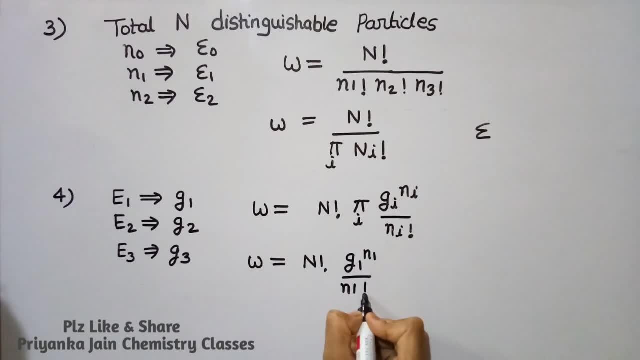 power n1 divided by n1 factorial into n factorial. g2 to the power n2 divided by n2 factorial into g3 to the power n3 divided by n3 factorial. In this way we have to find out the number of ways, Okay. Okay, Now we have to find out the. 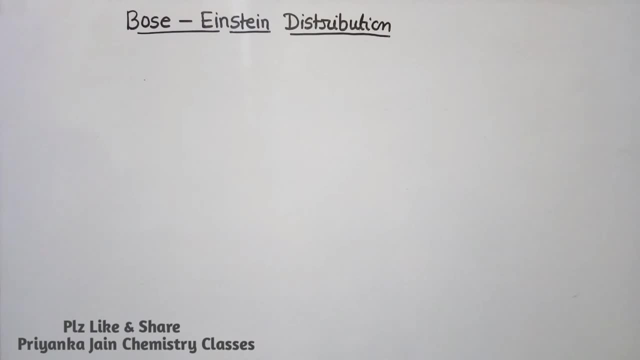 number of ways. in the case of the Bose-Einstein distribution, It means when we have given the particles that follow the Bose-Einstein statistics, It means particles are here. Firstly, the particles are indistinguishable, And another thing is that there is no restriction on the particles. Okay, These two conditions. 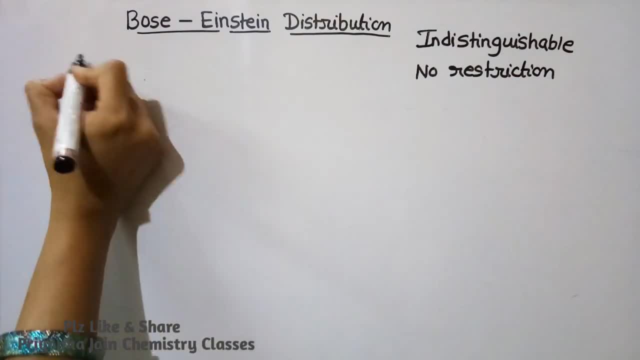 we must remember. Okay, Suppose we have given the number of particles is n. Okay, n is equal to 3 and number of states is m. Okay, We are denoting number of states by m and number of particles by m. So we have given the number of states by m. So we have given the number of. 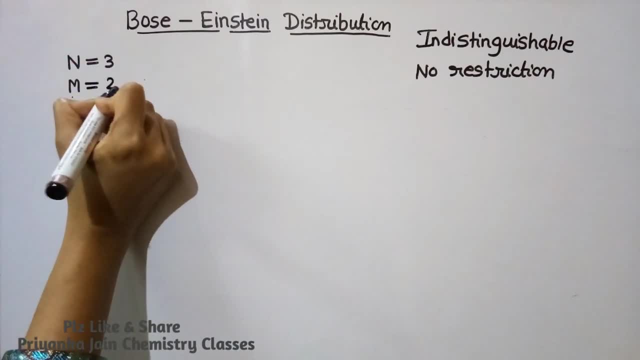 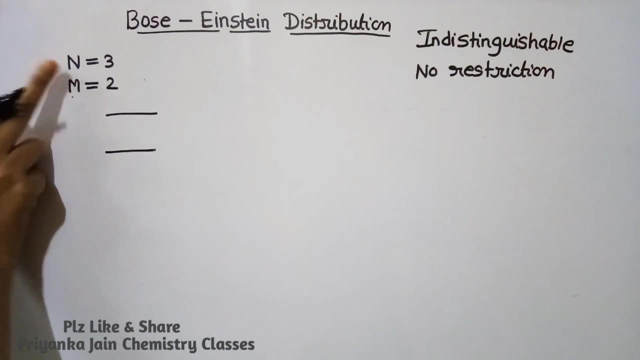 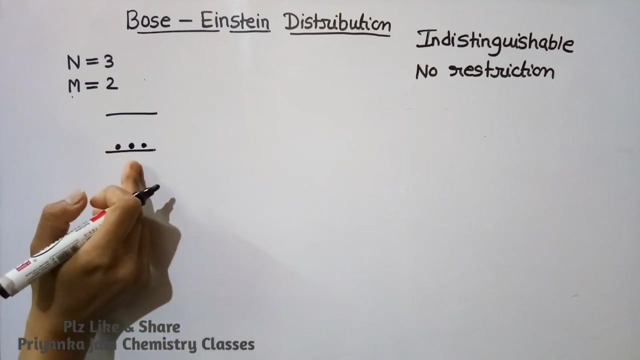 by n, okay, and M, is suppose it is 2, okay. so now see what can happen here. these are the two energy levels. okay, now see here, these three particles are indistinguishable. it means we cannot identify them. so these are three particles, okay. these can occupy one energy level. one condition is that? okay. 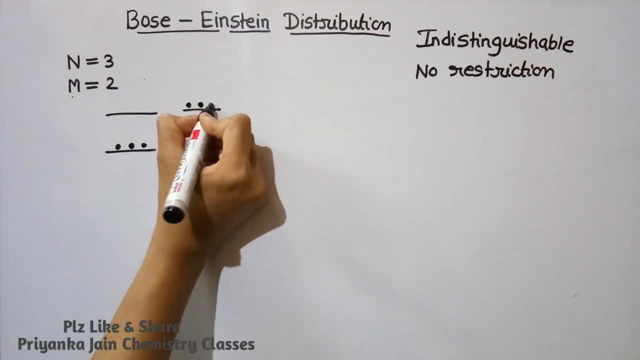 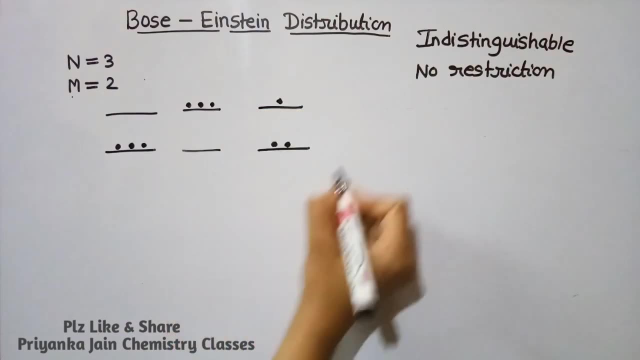 another condition may be that these three particles are present in this level right. third condition may be: two particles are present here and one is present here right. and the fourth condition is that these- there is one particle here and two particles are present here. okay, these are the four. 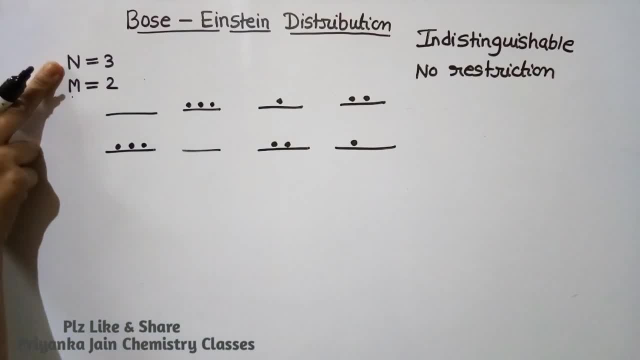 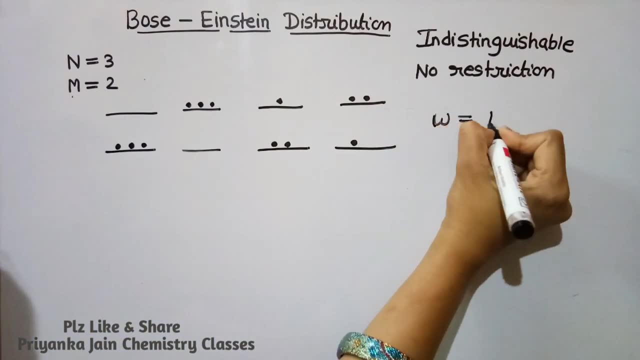 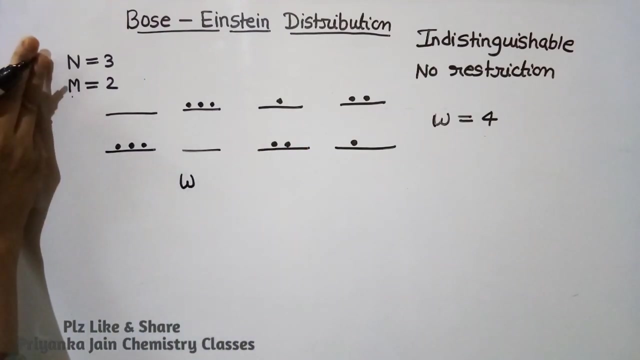 different ways in which we can distribute these three particles in that two energy levels. according to the Bose-Einstein statistics it means W is here equal to 4. so if we have to find out this by the formula, what is the formula for this if we have given so many number of the particles and so many? 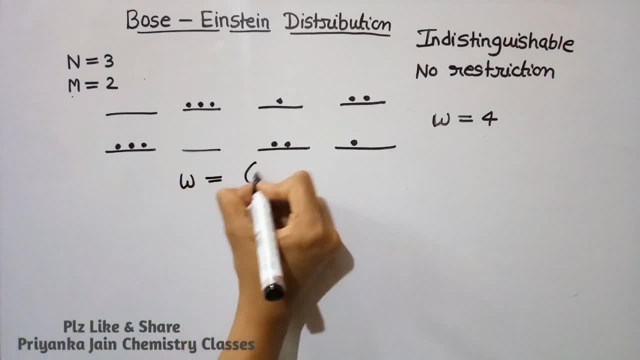 states. then formula will be: W is equal to n plus M minus 1 factorial divided by: firstly, write down here: n factorial- okay, n factorial. and M minus 1 factorial- okay, in this way we have to do, suppose we are seeing this condition. then here n is. 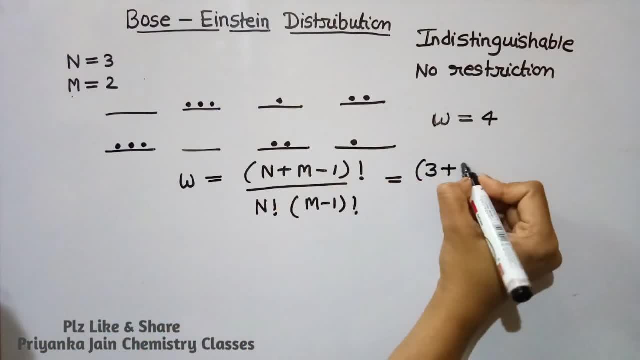 equal to 3. so 3 plus M is equal to 2 minus 1 factorial. divided by this is- we are seeing this condition then here: n is equal to 3 factorial and this will be: 2 minus 1 is equal to 1 factorial. okay, so if we are calculating is, this will be 3. 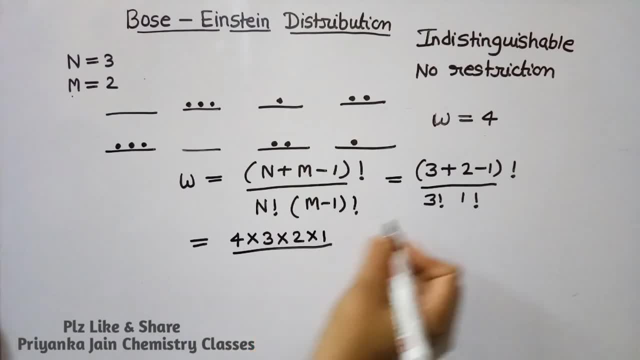 plus 2, 5, 5 minus 1, 4, so 4. factorial, it means 4 into 3 into 2 into 1. okay, and here will be this: 3 into 2 into 1, right, so what we are getting? we are getting. 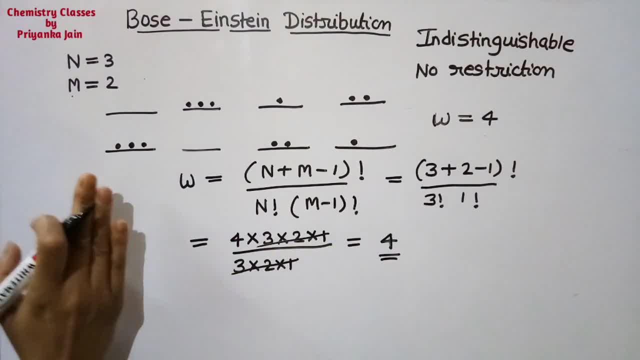 this will be cancel out. okay, we are getting 4 ways, so number of ways equal to 4. okay, another condition is here, when we have given the degeneracy. okay, Suppose ni is the any state and its degeneracy is gi. okay, So what will be the formula here? Formula will be: w is equal to pi i. 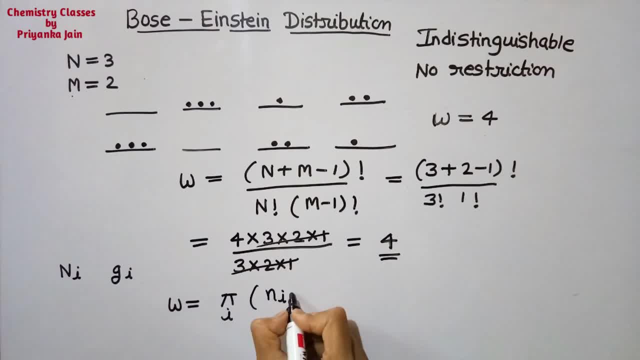 ni plus gi minus 1 factorial divided by ni factorial gi minus 1 factorial, It means we have to take all the molecules in the similar way and we have to multiply them. okay, Suppose we have given n1,, n2, another. So we have to write down here all the terms and we have to 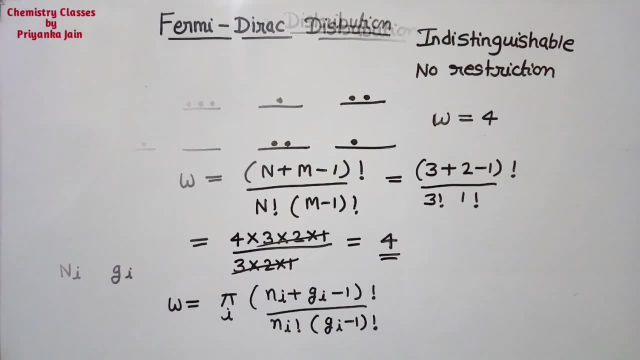 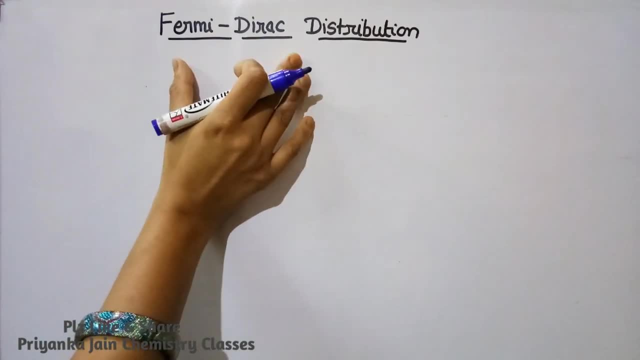 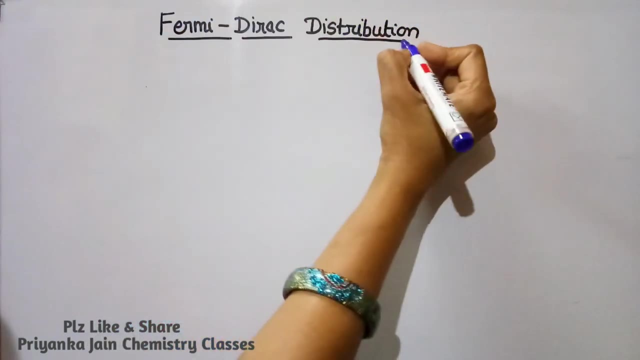 multiply them right In this way. we have to do this. okay. Now see the another thing. That is the distribution of the particles according to the Fermi direct statistics. It means we have to find out the number of ways when the particles are obeying the Fermi direct statistics. Now in this, 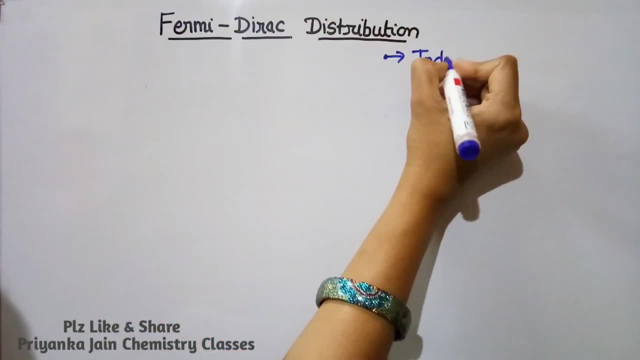 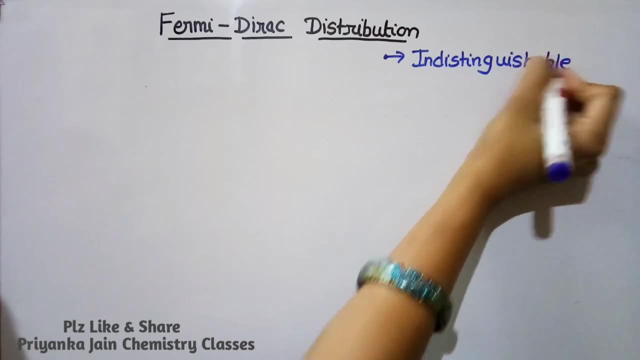 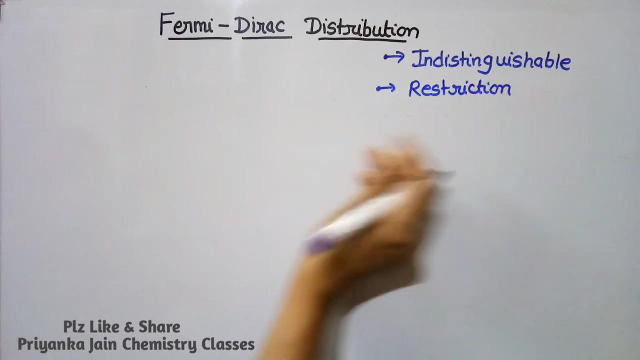 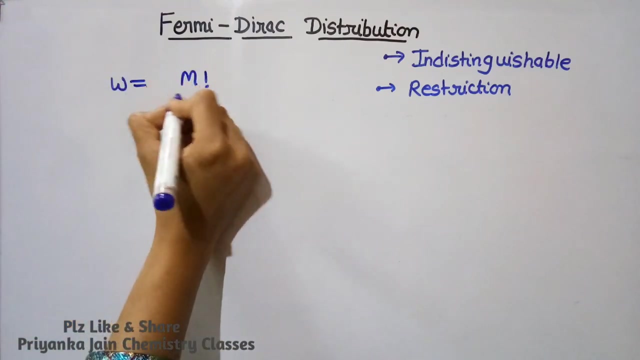 what is the criteria? The criteria is that the particles are indistinguishable and there is restriction on the particles. okay, This is the one important thing, Because here is the restriction on the particles. It means one particle can occupy only one energy level. right, So now, here see the formula. Formula is: w is equal to m factorial divided. 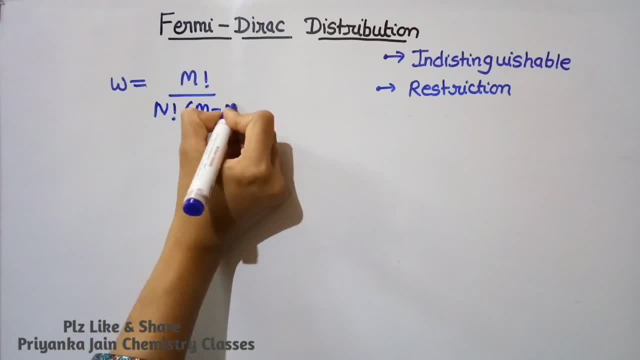 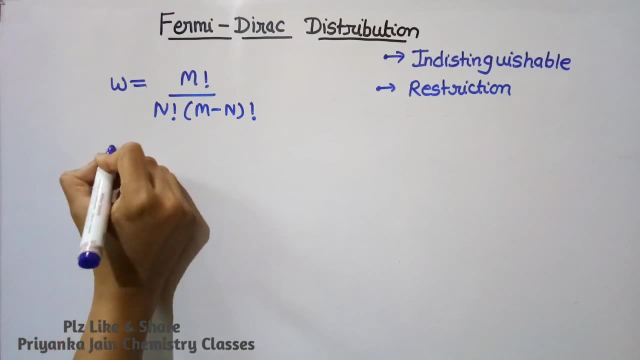 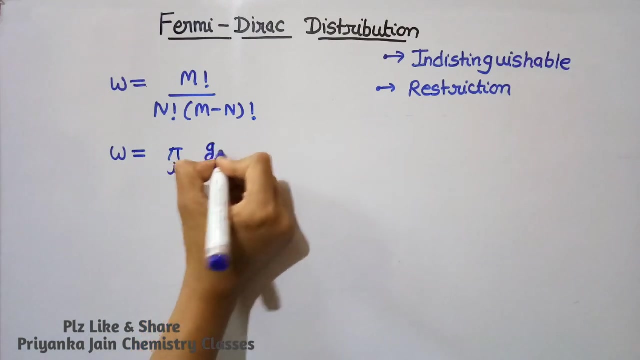 by n factorial, m minus n factorial- okay. And if we have given the degenerate states, it means the degeneracy is given to us. Then the formula will be here: w is equal to multiplication of all the terms gi- factorial divided by ni factorial, gi minus ni factorial- okay, These 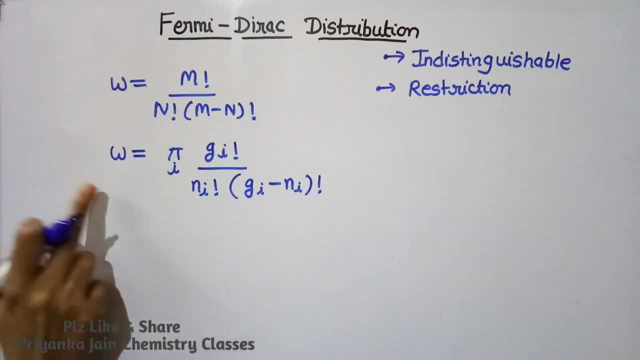 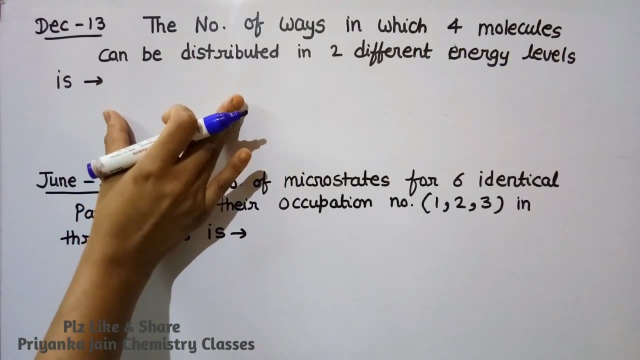 all formulas we can understand with the help of the examples. So I am giving you the examples that has been asked in the net and the get exam, okay, Okay, now see from the simplest case okay Towards the complicated cases. Firstly, we 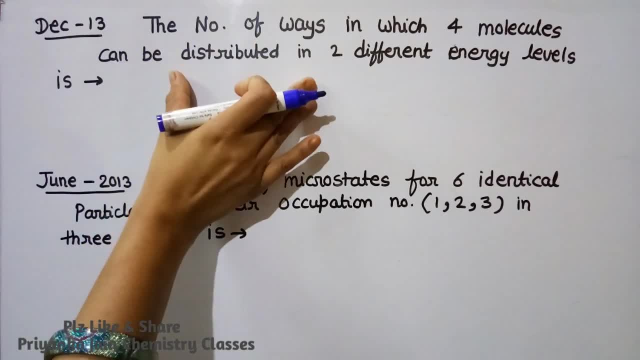 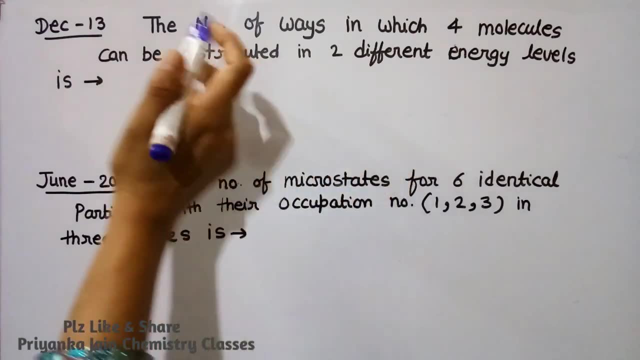 are seeing the simplest question from December. Here we have given a general question. The number of ways in which 4 molecules can be distributed in 2 different energy levels is okay. So here n is equal to 4 and m is given. 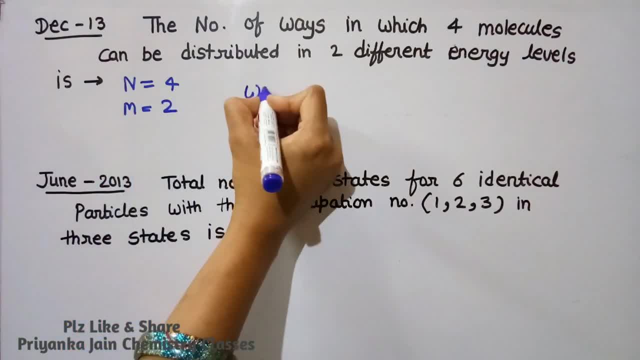 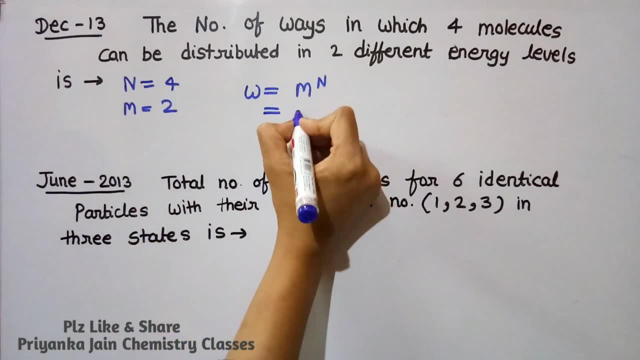 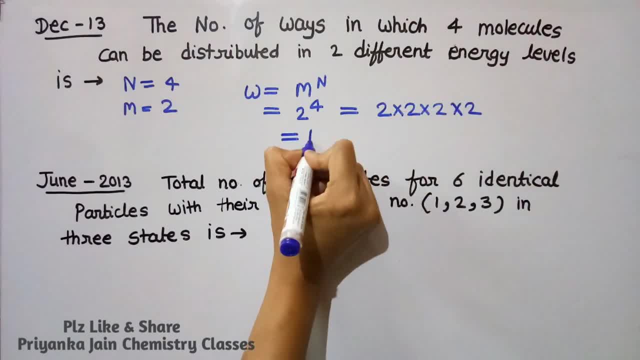 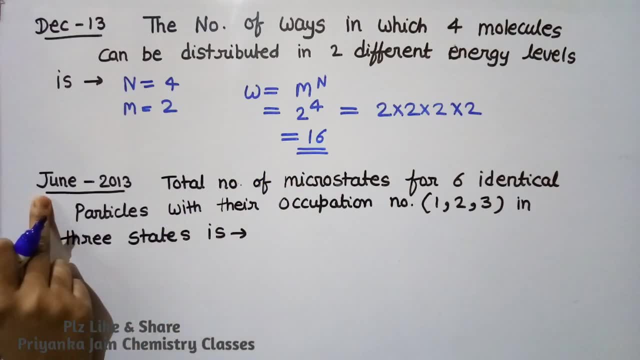 2 into 2 into 2.. So it will be equal to 16.. It means there are 16 ways of distributing particles. okay, Now see this question from June 2013.. The question is: total number of microstates for 6 identical particles with their occupation number 1, 2 and 3 in 3 different. 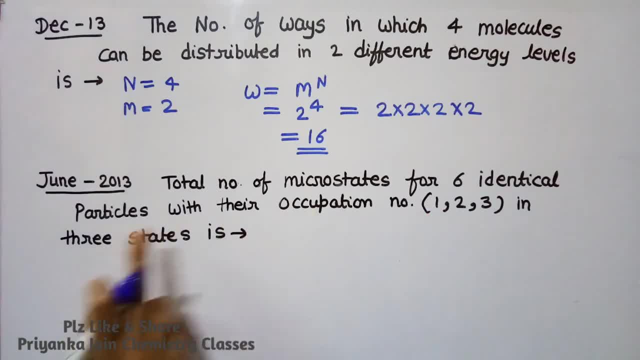 states. It means 1 particle is in 1 state, 2 in another state and 3 in the third state. okay, So total number of particles is here 6.. And what will be The formula I have already told you Here? we have to write in this way: Total number. 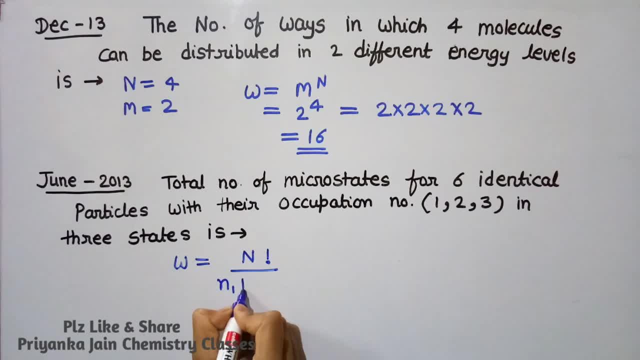 of particles, factorial, and then n1 factorial, n2 factorial, n3 factorial. okay, In this way we have to do here, So write down here: number of particles is 6.. So 6 factorial divided by 1 particle is present in 1 state, 2 particles are present in another state and 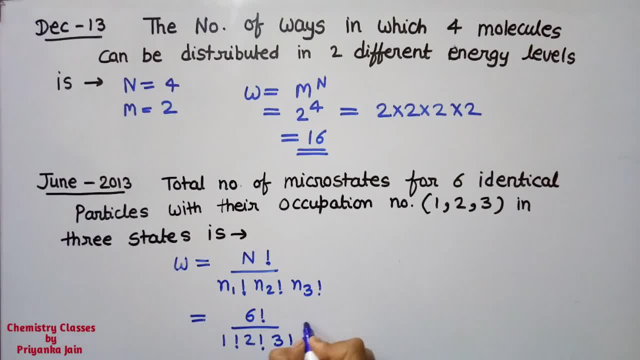 3 particles are present in the rest state: okay. So if we are calculating this one, 6 into 5, into 4, into 3, into 2, into 1, okay, Divided by this is 1, okay, This is 2.. So 2 into 1 and this is 3, 3 into 2 into 1, okay. So this will. 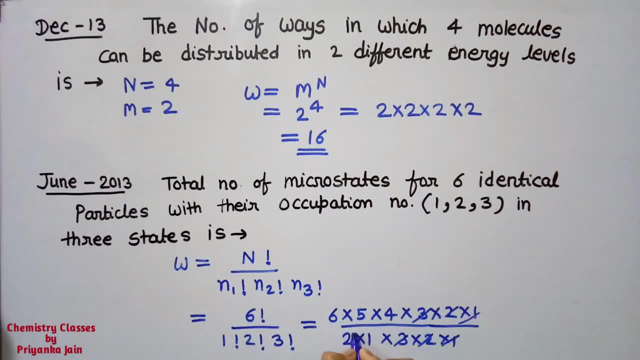 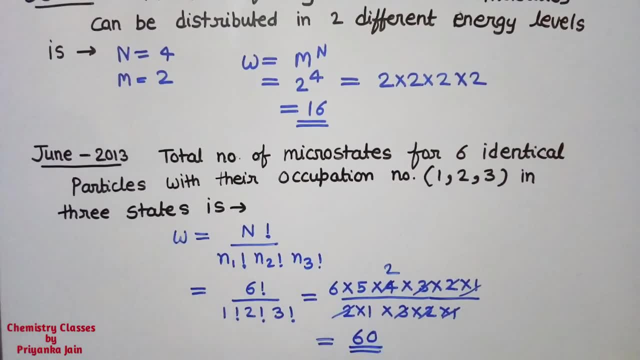 cancel out. Now this is 2, okay, So we are getting here 2.. So this will be equal to 60, okay, So there are 60 ways or 60 ways of distributing particles. So this is 2. 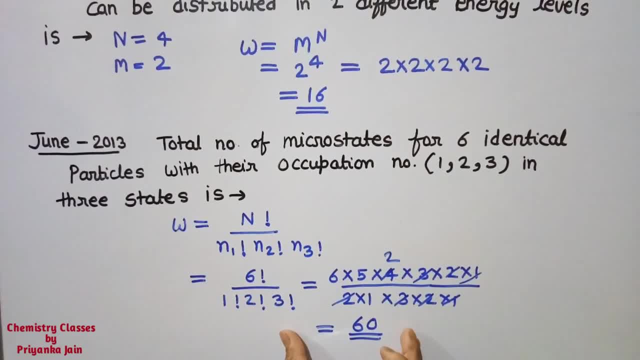 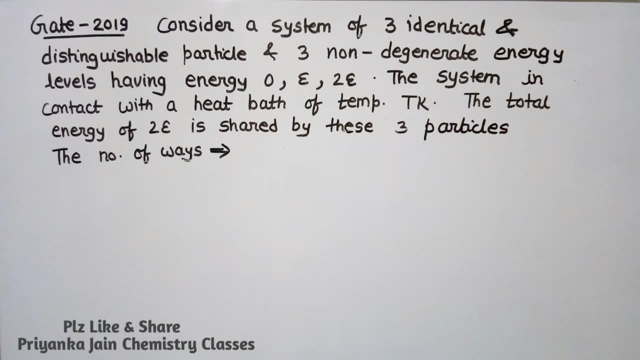 ranks of 60 microstates for distributing particles. okay, Let's see this question from GATT 2019.. The question is: consider a system of 3 identical and distributable particles and 3 non-descended energy levels, having energies 0, E and 2E. 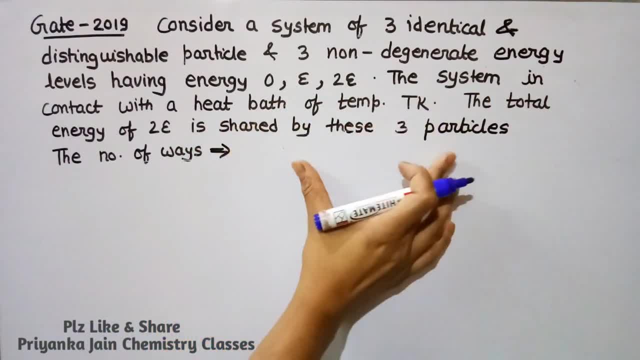 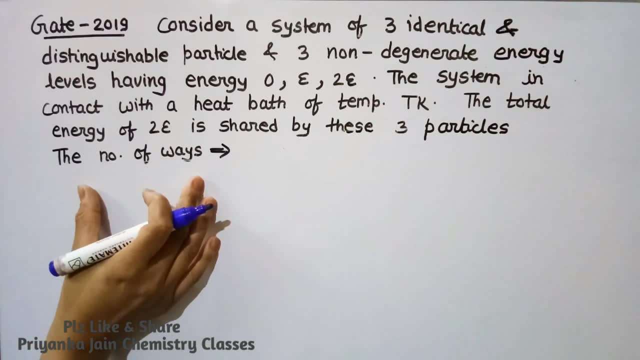 okay, The system in contact with a heat path of temperature, T Kelvin. the total energy of 2E is shared by these 3 particles, and now we have to find out the number of ways. First thing that we have given is v, e, e, e and e, So 2e is equal to 0, e, e 1, e, 2, e. 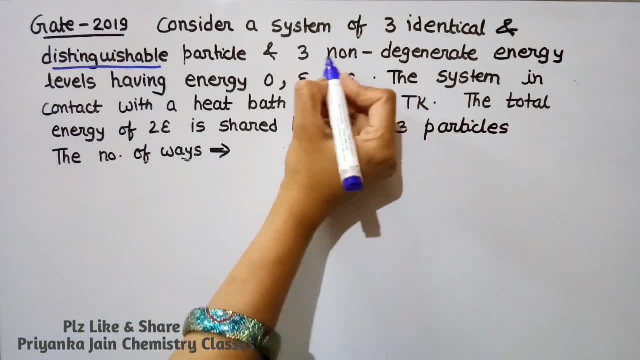 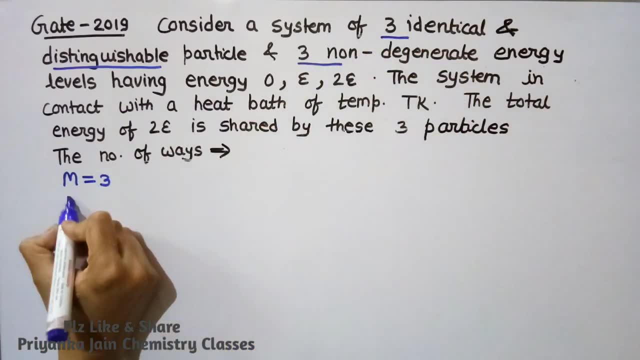 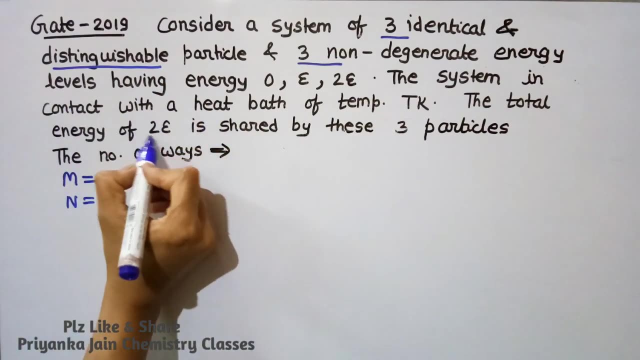 given is that the particles are distinguishable. okay, And there are 3 energy states. It means the value of m is equal to 3, okay, Number of particles are 3 and that are distinguishable. right Now we have to distribute this energy in this way that the total energy is equal to 2e. 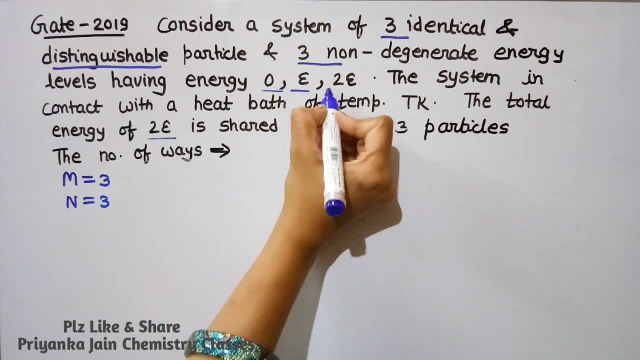 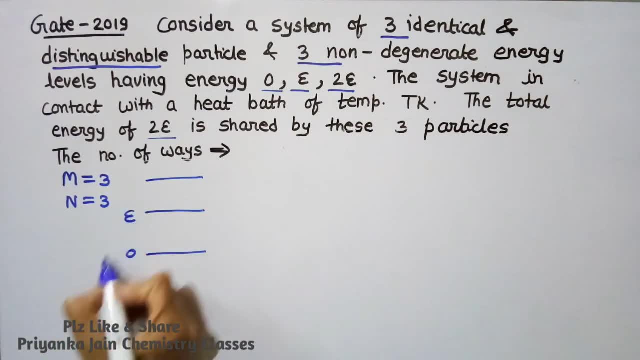 and the energy of these 3 labels is 0,, e and 2e. It means if we are making 3 energy labels in this way, this will have 0 energy, this will have e energy and this will have 2e energy. 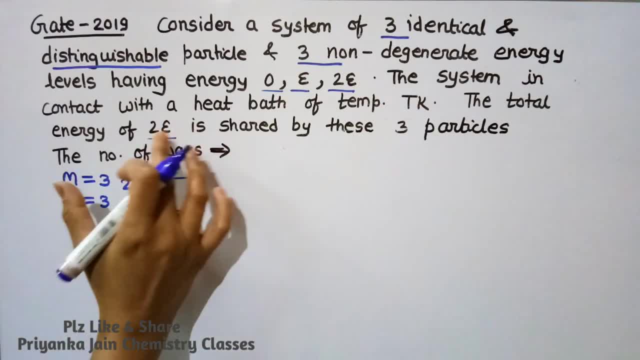 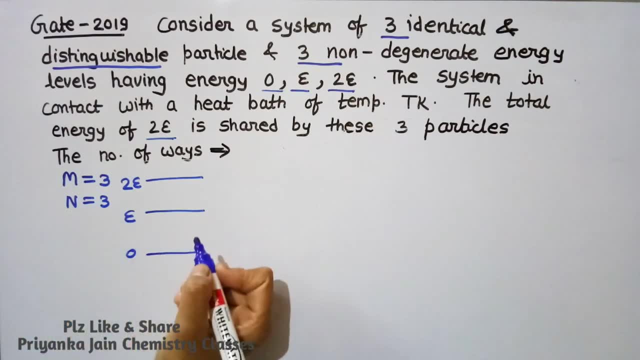 And now we have to distribute the particles in such a way that the total energy is equal to 2e. okay, All the things are now clear. okay, Now particles are distinguishable, so we can represent them by a, b and c. okay, So one condition is that that the both particles 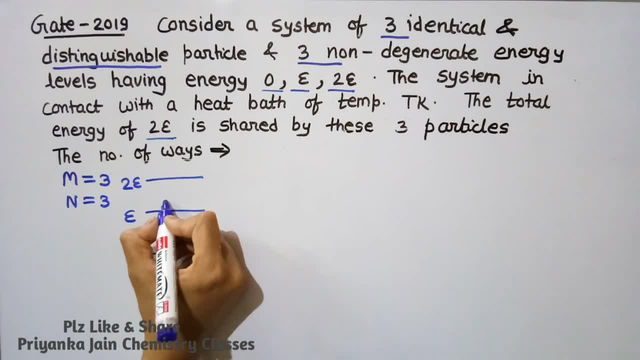 are present in this e label. okay. One condition is this: and the rest particle is present in this e label, okay. So one condition is that that the both particles are present in this e label, so the total energy will be equal to 2e. okay, There may be 3 condition of such type. 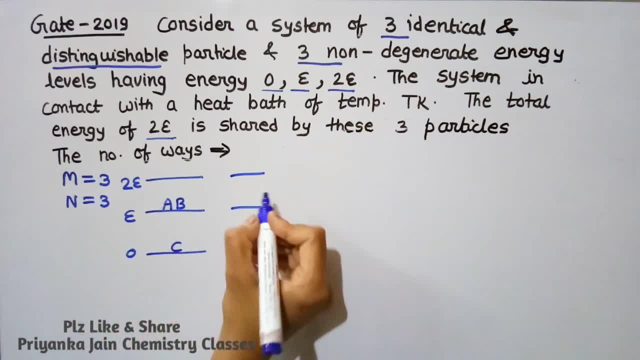 because the particles are distinguishable, we can identify them, okay. So one condition may be that b, c are present here and a is present here, right. And the third condition may be that here b is present and a and c are present here, right. Okay, now there may be another, different way. 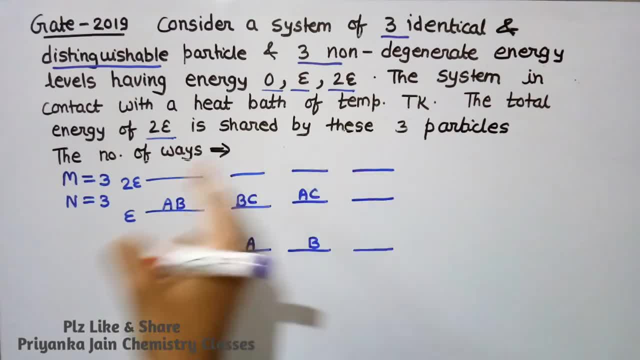 What is the way That one particle is present in this 2e label? Suppose a is present here and b, c are present here. okay, Then the total energy is equal to 2e. So there may be 3 condition of the similar type. One is that b is present here and c and a are. 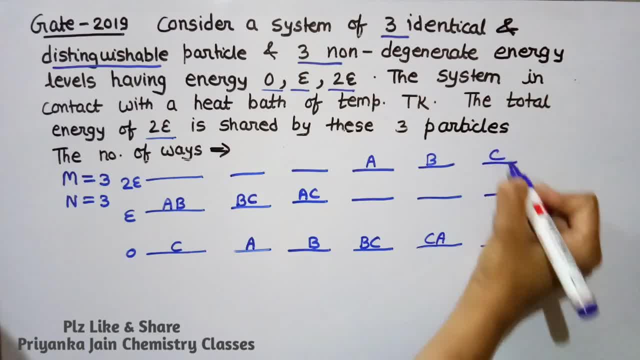 present here and the another condition is that c is present here and a and b are present here, right? So these are the 6 ways in which we can distribute these 3 particles among these 3 energy labels. okay, So the number of way is equal to 6.. This is the answer of this question. 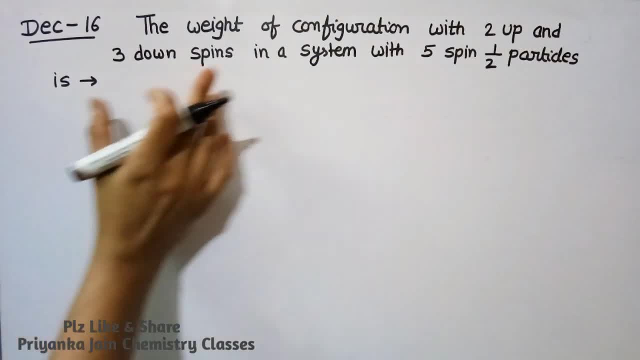 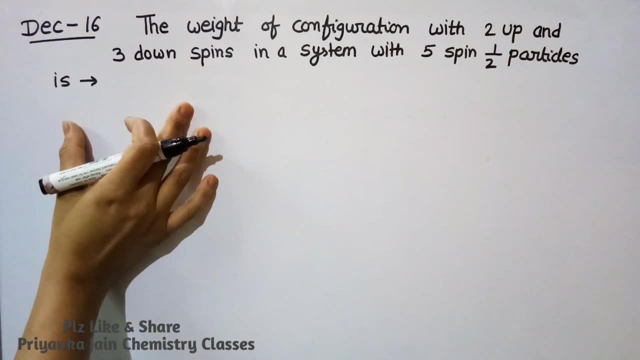 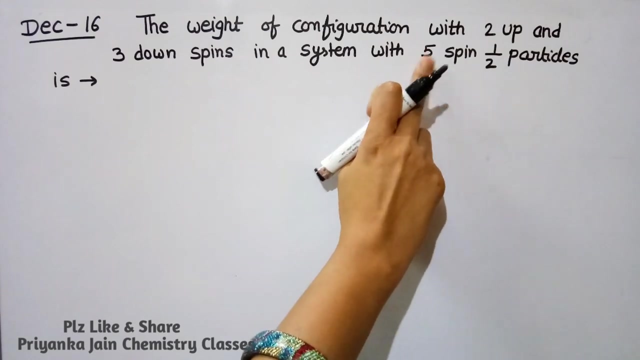 Okay, now see this next question from December 2016.. The question is the weight of configuration with 2 up and 3 down spin in a system with 5 spin half particles. is It means we have given spin half particles or we have given the fermions right And total number of particle is equal to? 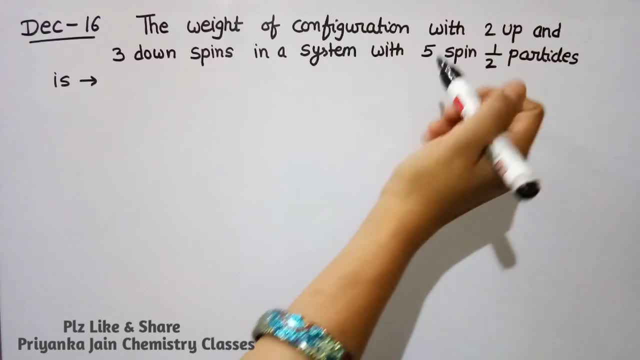 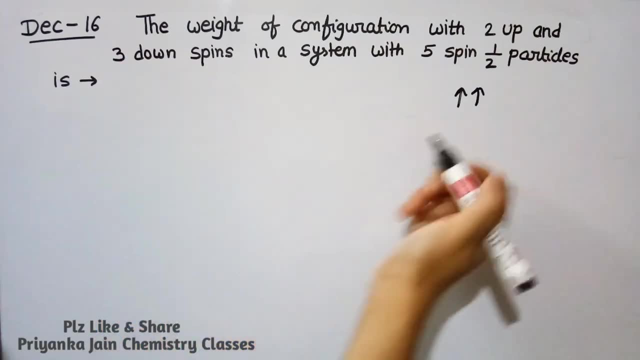 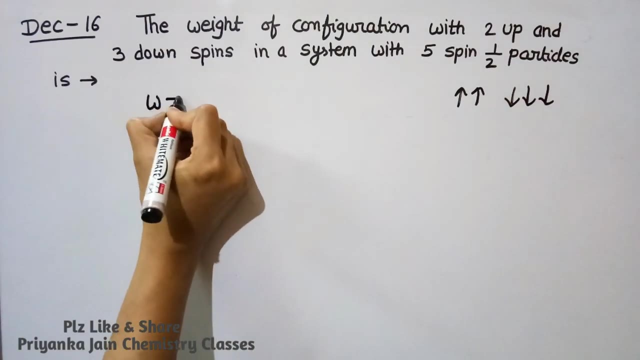 5, right, And there are 2 different states. One state is when the 2 particles are upside. it means in this way, upward spin, okay, And 3 will have the downward spin. The another state is: this one right. So these are the 2 states. So the number of ways is given by total number of. 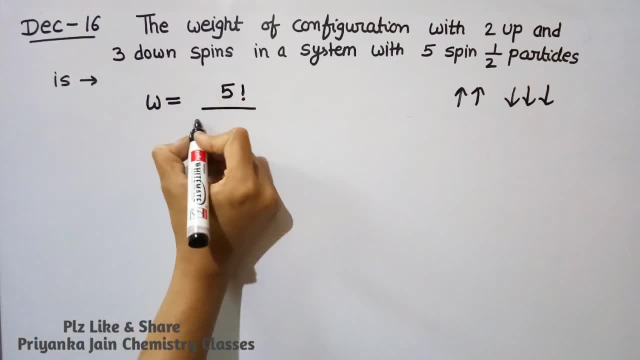 particle is 5.. So 5 factorial divided by 2 are present with the upward spin and 3 are present with the downward spin. in this way, right? So 5 into 4, into 3, into 2, into 1, divided by 2, into 1. 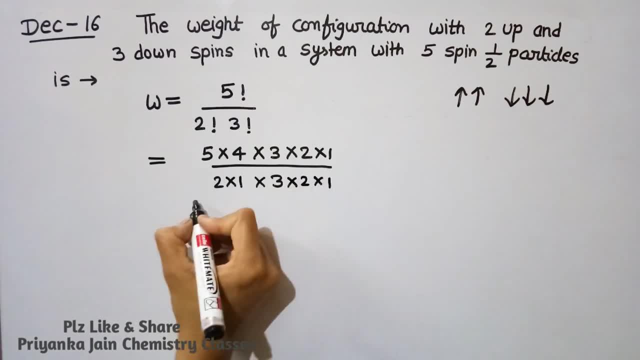 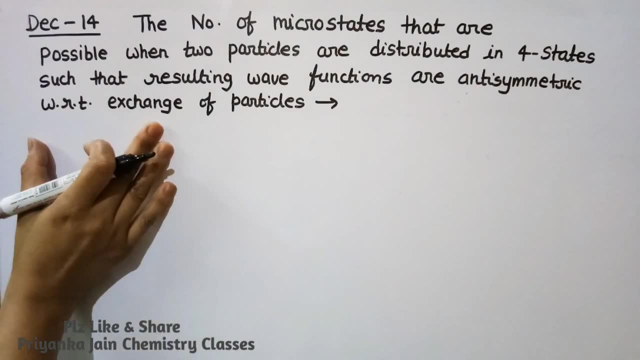 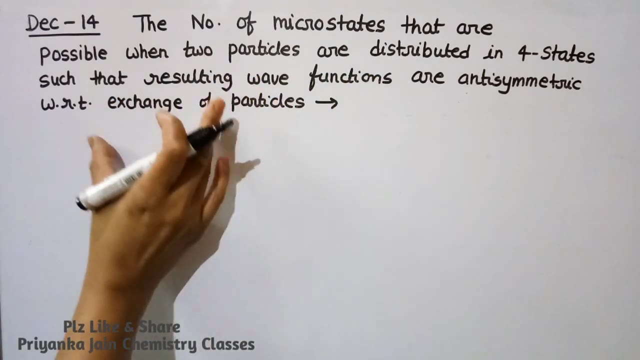 into 3, into 2, into 1, okay, So there are 10 ways. Next question is from December 2014.. The question is number of microstates that are possible when 2 particles are distributed in 4 states, such that the resulting wave functions. 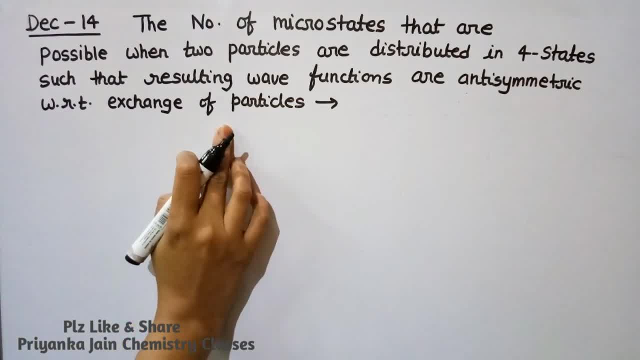 are antisymmetric with respect to exchange of particles. okay, So here one thing: we have, given that the resulting wave function is antisymmetric with respect to exchange of particles, It means the particles are fermions, Okay. Another thing: number of particles is 2 and the number of states is 4, okay, And we have to. 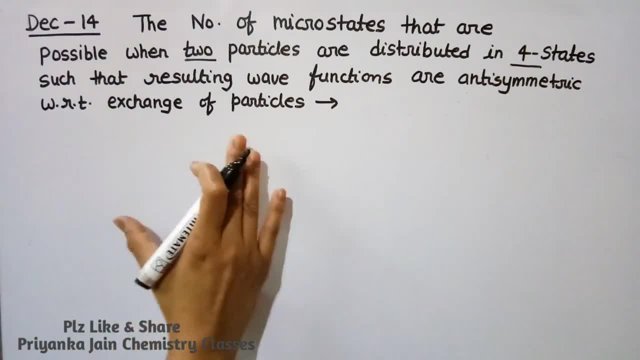 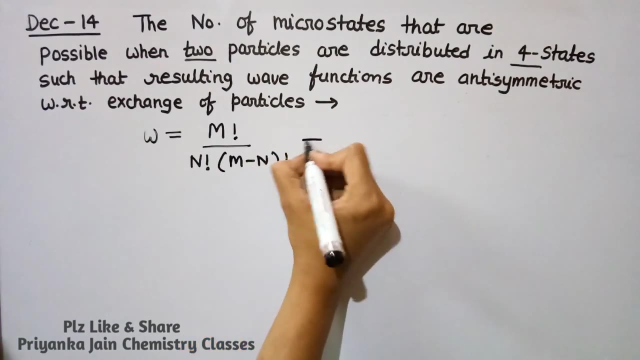 find out the microstates, or we can say number of ways. Both the things are same, okay, So don't confuse. So w will be equal to. just we have to apply the formula of fermions. What is the formula? m factorial divided by n factorial, m minus n factorial? okay, And just we have to put the 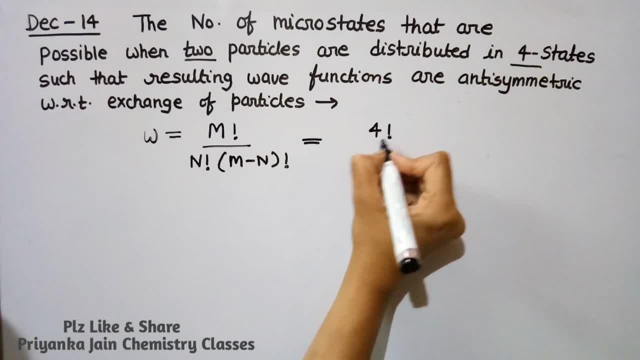 values. What is the value for m? That is equal to 4, okay. So 4 factorial divided by number of particles, 2, 2 factorial, and 4 minus 2 is equal to 2.. So 2 factorial. So what we are getting now. 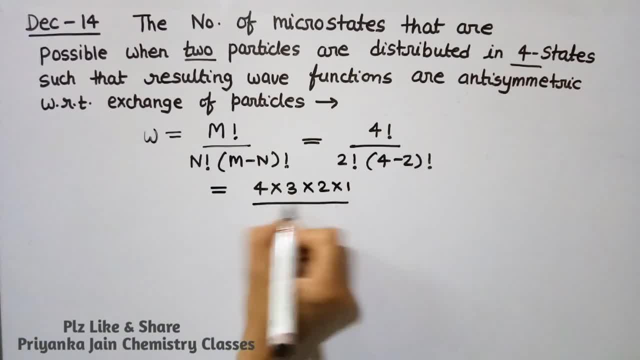 4 into 3 into 2 into 1, divided by 2 into 2,. okay, So this will cancel out and number of ways will be equal to 6.. It means total number of microstates are here 6,. okay, This is the answer. 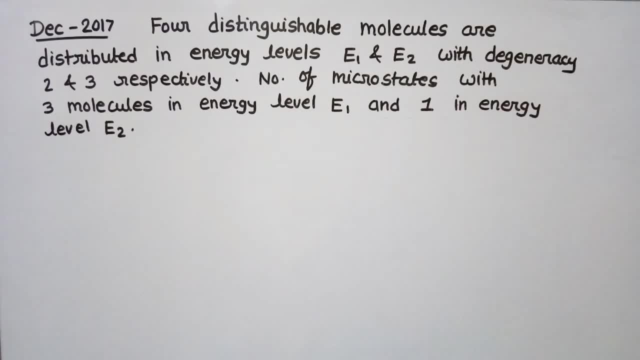 Let's see this question from December 2017 and very important question. see here: 4 distinguishable molecules are distributed in energy levels E1 and E2, with degeneracy 2 and 3 respectively. okay, Degeneracy is 2 and 3, okay. Number of microstates with 3 molecules in the energy level E1 and 1. 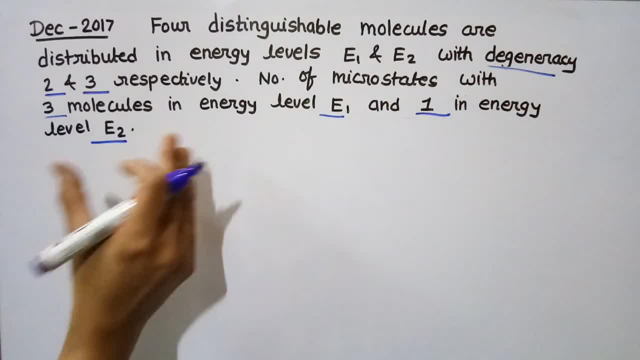 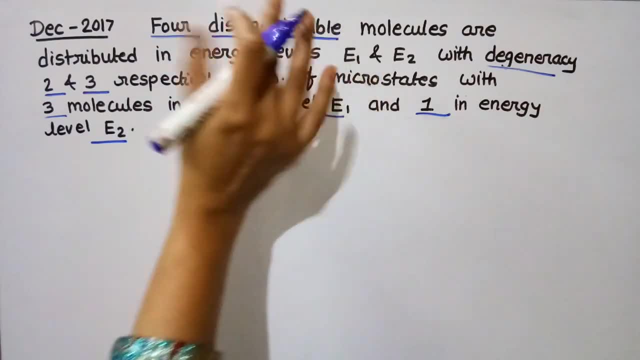 molecule in the energy level E2,. okay, So we have to find out here the number of microstates, right? Total number of particles is 4 and we have given distinguishable particles. It means we have given here the max valence, okay. Okay, So total number of particles is 4 and we have given here. 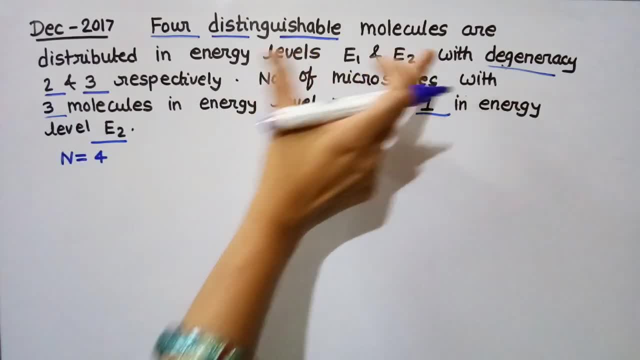 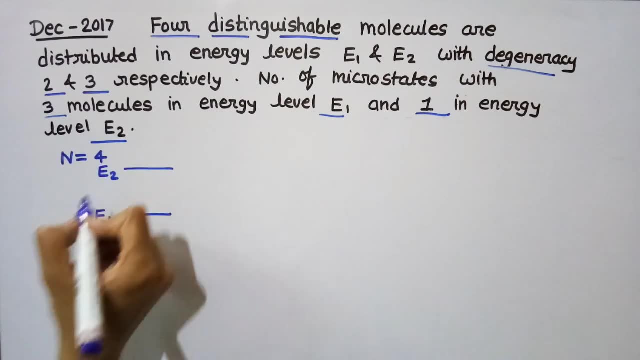 the max valence. okay, So total number of particles is 4 and we have given here the max valence, right. And there are 2 energy levels: One is E1 and another one is E2, right, And now what is said? 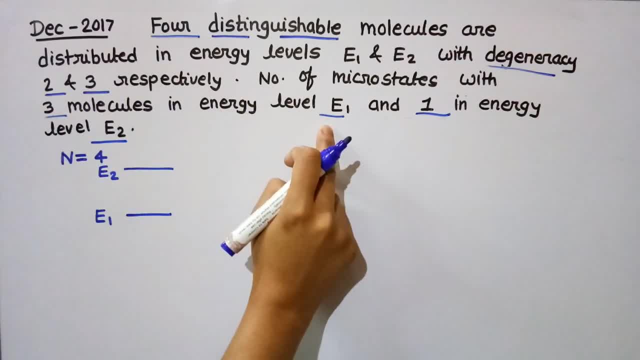 here that 3 molecules are present in the energy level E1,. okay, So N1, this will be N1.. N1 is equal to 3, okay, N1 is the number of molecules in this level: E1 and N2, it means number of. 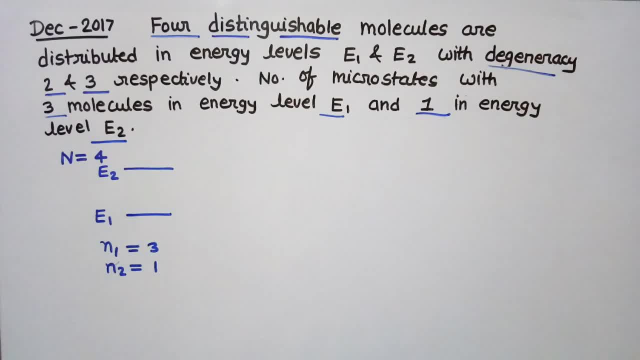 molecules in this level, E1.. So N1 is equal to 3, okay, So N1 is equal to 3, okay, So N1 is equal to 3,. molecules in this level E2 will be equal to 1.. Now, what thing we have given degeneracy. It means 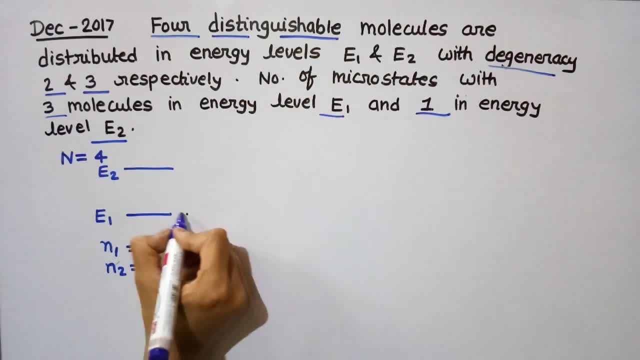 the degeneracy in the case of this level, E1,. in the case of E1, the degeneracy is equal to 2, and in this case, the degeneracy is equal to 3,. okay, Now, what formula we have to apply here? 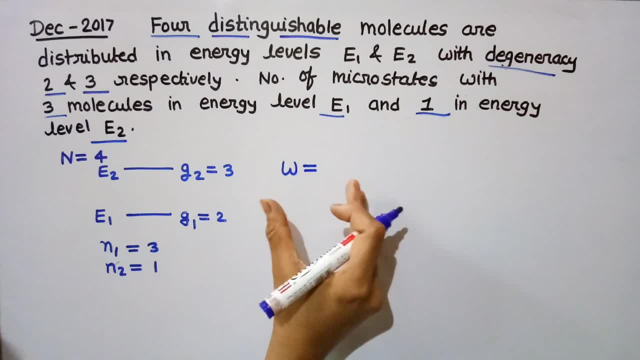 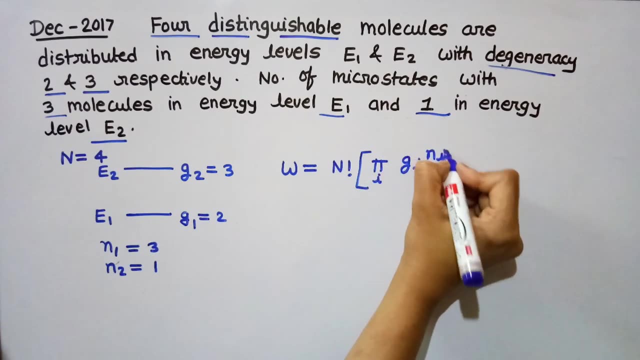 I have already told you one formula for the Maxwell-Boltzmann statistics That includes degeneracy term. What was that? n factorial. then multiplication of all the terms: g, i to the power: n i divided by n i factorial. okay, we have to apply just this formula. so see here: total number of particle.